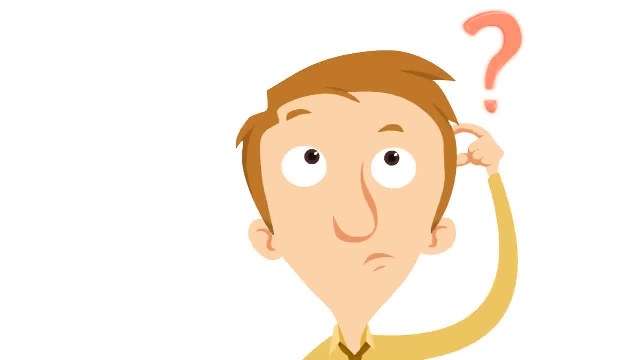 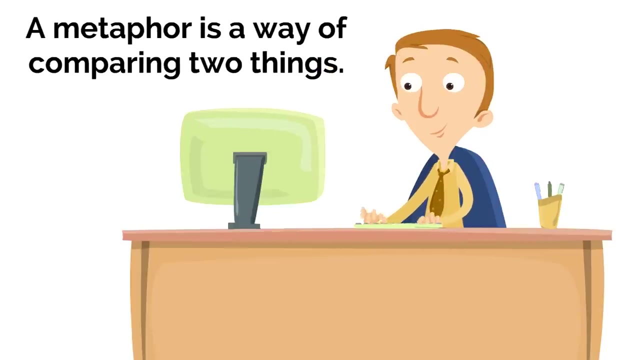 how to use them. First, what is a metaphor? What is a metaphor? Well, a metaphor is a way of comparing two things. It's not the only way to compare two things, but it's a very interesting and creative way of comparing two things. 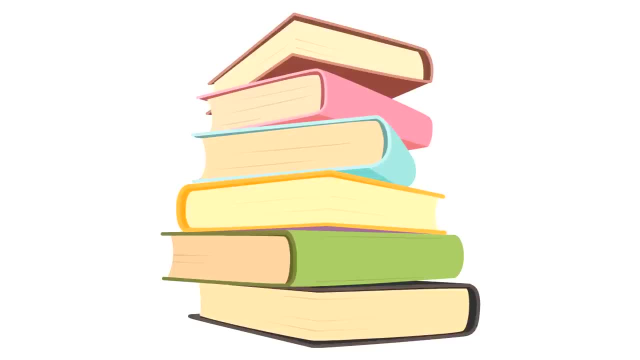 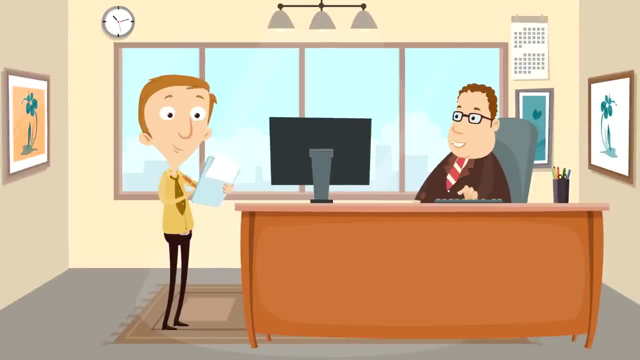 You might have seen examples of metaphors and books and in poetry, and there's a really big chance that you use metaphors in your everyday speech as you're speaking to people. we just use metaphors from time to time and Bob loves using metaphors when he speaks to me. he loves comparing things in a 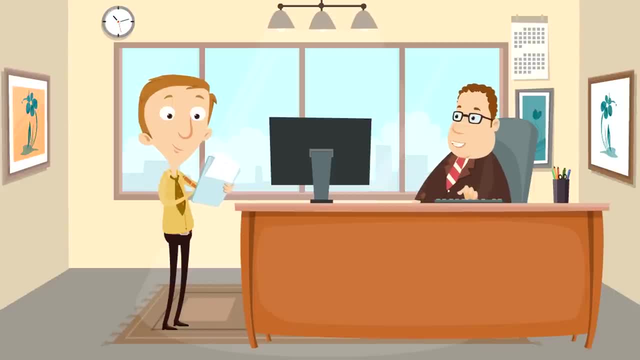 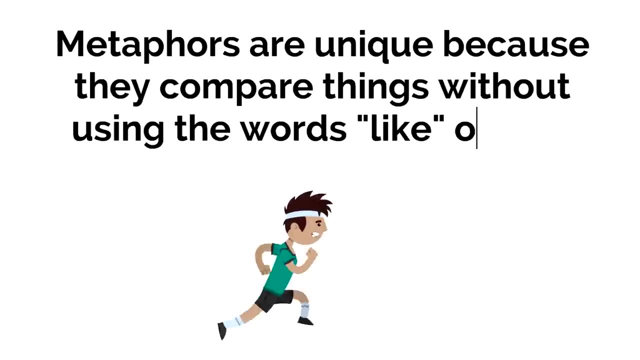 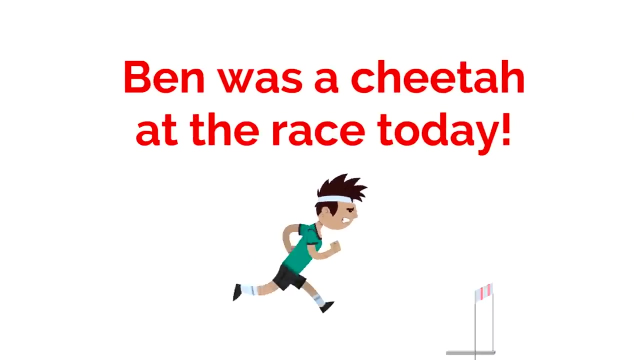 really creative way. metaphors are unique because they compare things without using the words like or as, and we're gonna look at some examples. at first they're going to look a little bit weird, but then you'll get the hang of it and you'll see how fun they are to use. here's an example: Ben was a cheetah at. 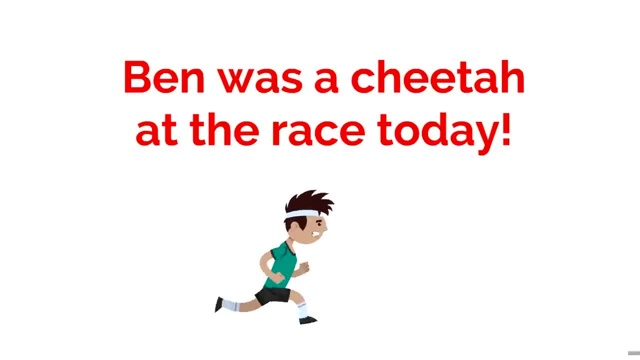 the race today. Ben was a cheetah at the race today. we are comparing in this sentence Ben to a cheetah because he went so fast. and cheetahs are not cheetahs, they are cheetahs. cheetahs are not cheetahs, they are cheetahs. 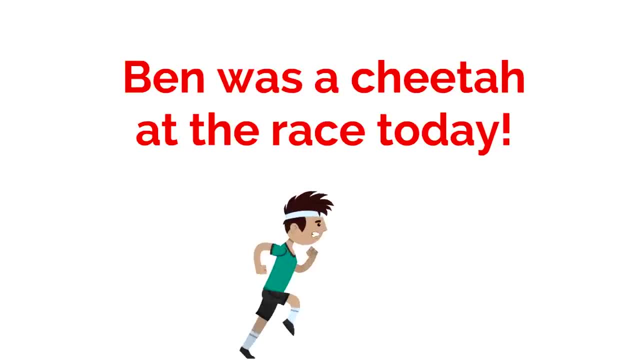 cheetahs are not cheetahs, they are. cheetahs are the fastest land animals in the world. so we're comparing ben to a cheetah. it's a metaphor, because we're making this comparison without using the words like or as. 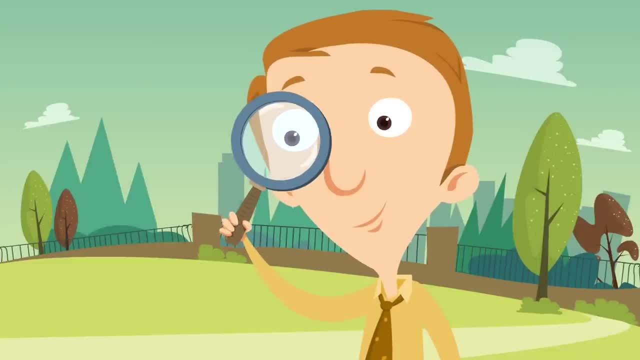 we mentioned earlier that metaphors can sound silly. that's because in our example, ben is not really a cheetah, even though we said ben was a cheetah at the race today. it's a way of comparing that makes it sound like there's no difference between them at all. 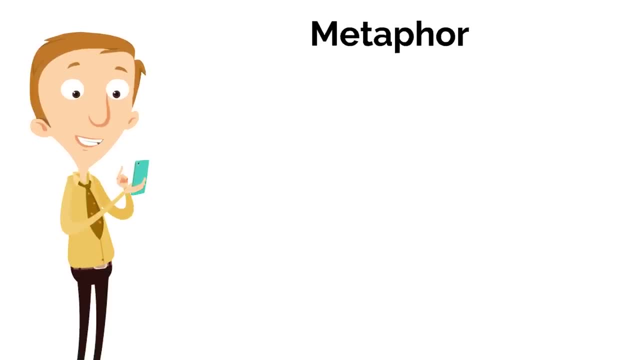 let's look at our metaphor again. ben was a cheetah at the race. today is a metaphor. it's comparing ben to the cheetah and it's not using the words like or as. okay, let's pretend we did use the word like or as. what if our example was: 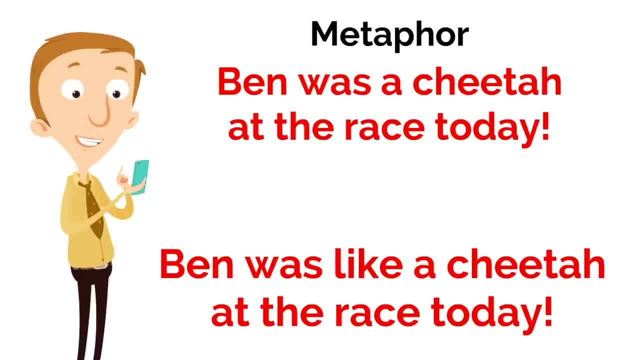 ben was like a cheetah at the race. today that makes it a different type of comparison, called a simile a simile. a simile is different than a metaphor because a simile makes a comparison using the words like or as. remember: metaphors are comparisons that. 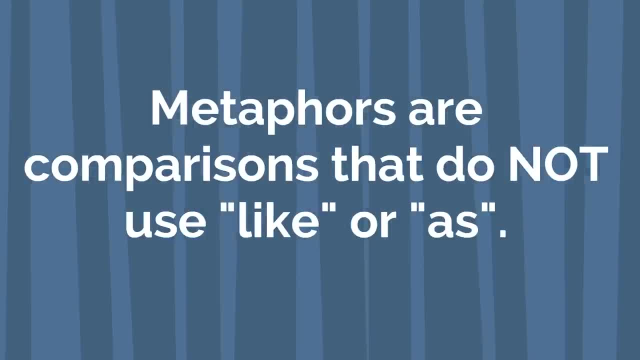 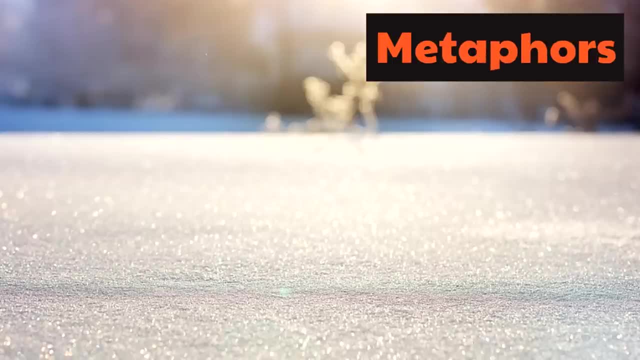 do not use like or as metaphors. metaphors are comparisons that do not use like or as. look at this example. the snow was a white blanket on the ground. the snow was a white blanket on the ground. in this metaphor, we are comparing the snow to a blanket. 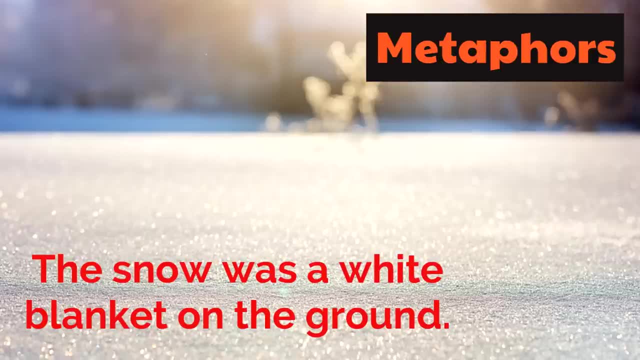 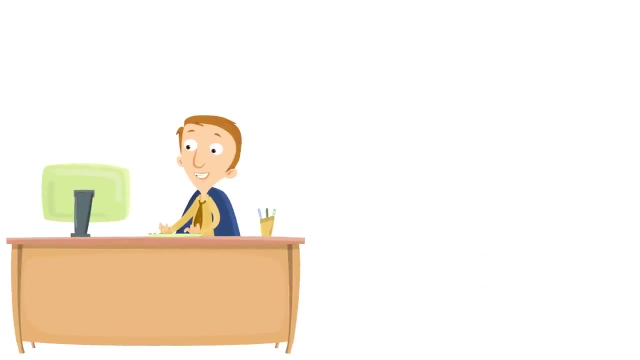 in this metaphor we are comparing the snow to a mountain. notice: you don't see the word like or as. this is definitely a metaphor, because it's a comparison that is not using the word like or as. let's think back to our examples. the first one, ben. 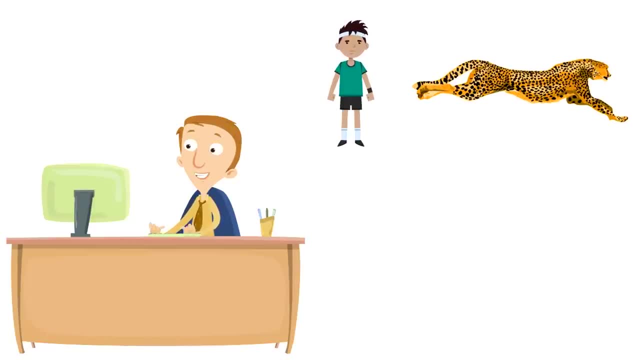 is compared to a cheetah and he is called a cheetah. the comparison doesn't use the word like or as, so that was a metaphor- a metaphor speaking to how fast fast Ben was running. In our second example, the snow was compared to a blanket. 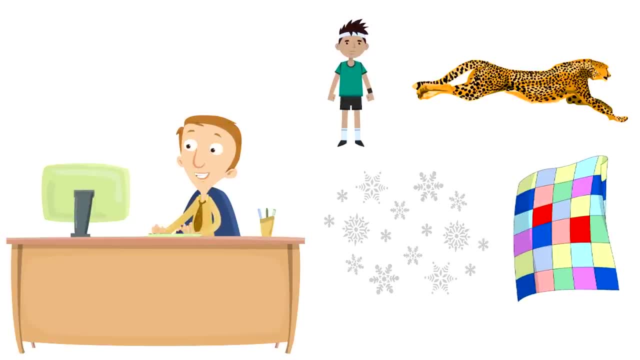 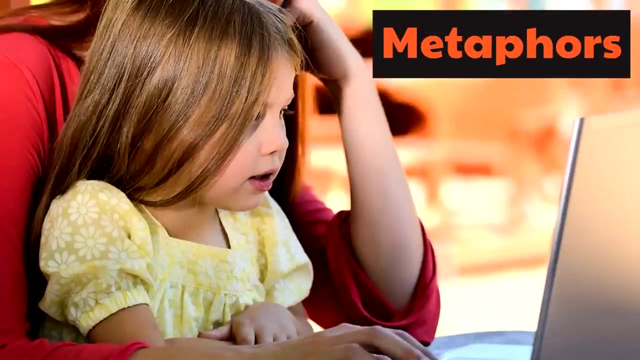 The metaphor said that the snow was a blanket on the ground. That's a comparison that is not using the word like or as. This second metaphor speaks to the appearance of the snow on the ground. Metaphors: A metaphor is a comparison that does not use. 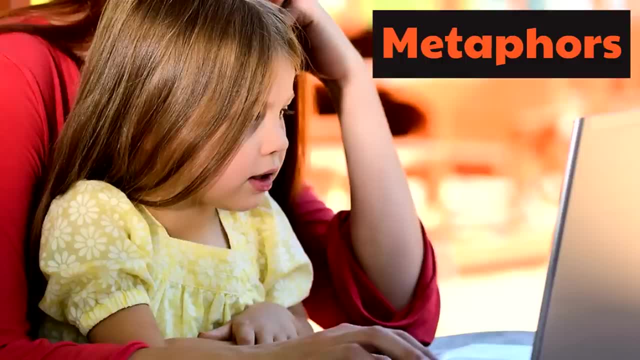 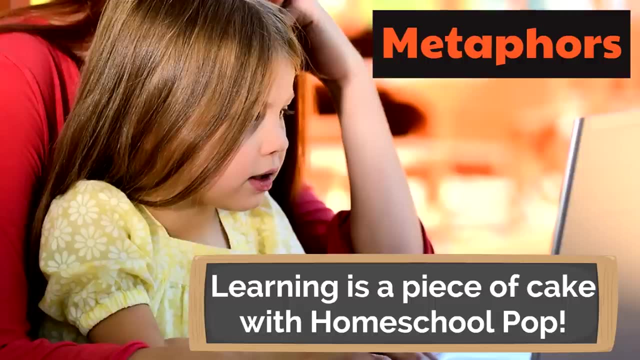 the words like or as. Look at this example: Learning is a piece of cake with homeschool pop. Learning is a piece of cake with homeschool pop. This is a metaphor Comparing the learning that you get with homeschool pop to cake, to a piece of cake. 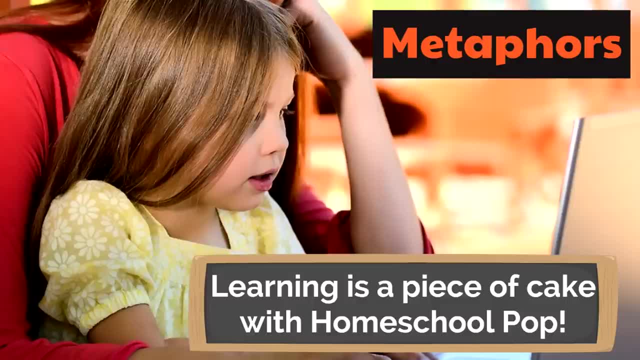 A piece of cake is a common metaphor speaking to how easy something is. Just like it's easy to eat a piece of cake, learning with homeschool pop in this example is easy. This is the metaphor. Learning is being compared to a piece of cake without using the words like or as. 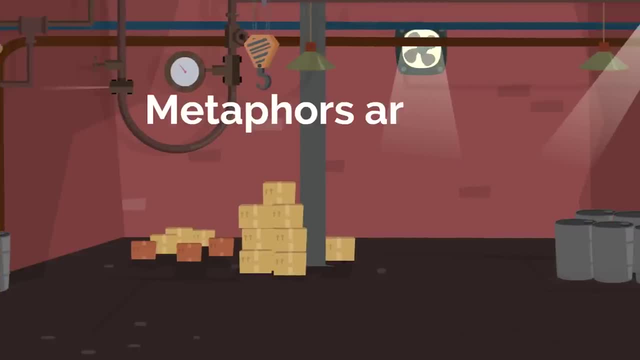 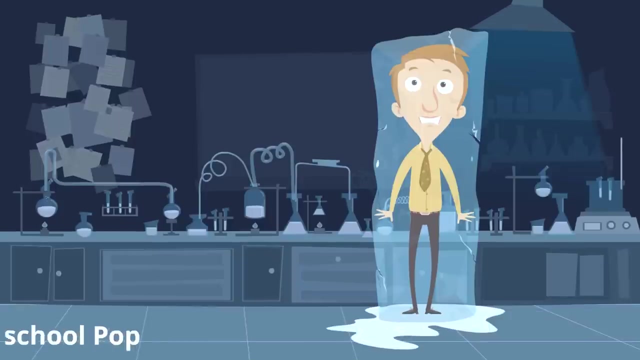 Metaphors are comparisons that do not use like or as. They're simple, they're fun and they are a creative way of comparing two things. I am a block of ice. No, that's not a metaphor. I'm not comparing myself to ice. 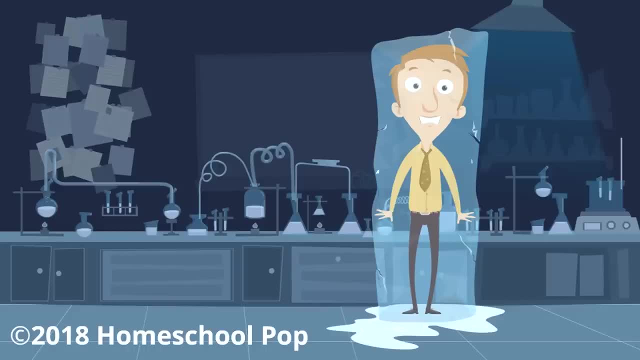 I'm frozen, okay, The big ice cube, Mr Whiskers, was in this lab with me. Mr Whiskers, Mr Whiskers, This ice is melting, It shouldn't take too long. Where's Mr Whiskers? 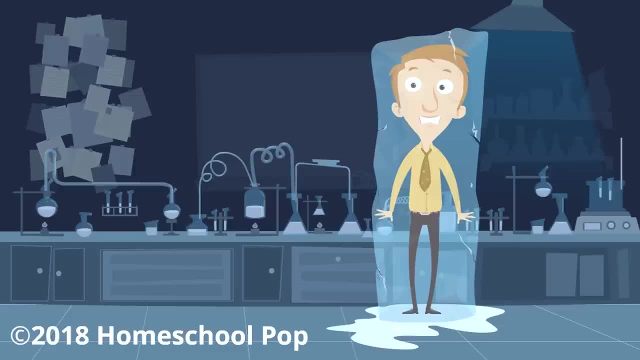 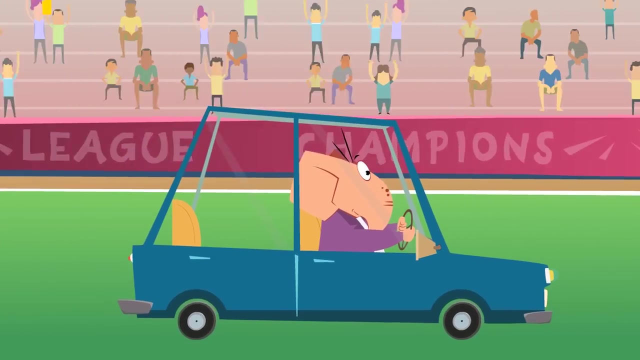 Where are you? Metaphors, a way of comparing two things without using like or as. but this is not a metaphor. I'm frozen, Hey, well, okay, first of all, elephants don't drive. okay, Elephants can't get a driver's license. 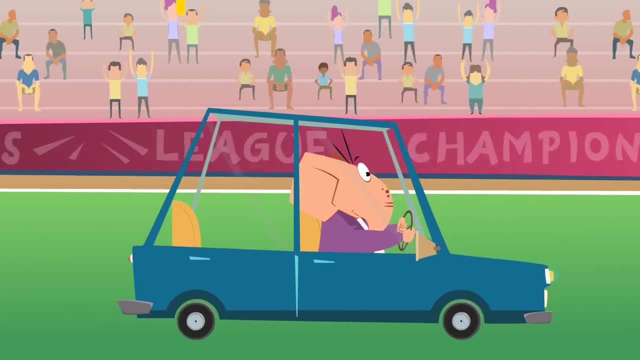 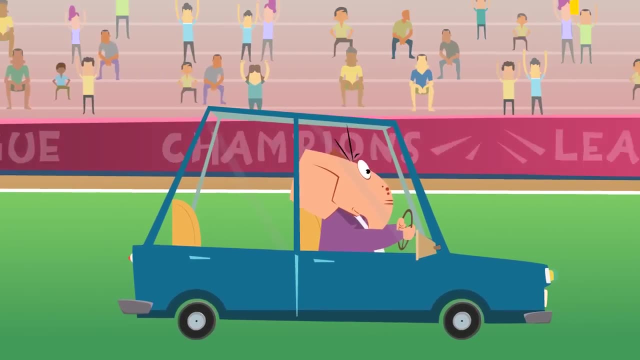 And he's driving on the grass. He's driving on the grass. You're going to ruin the lawn, okay. What's going on here? All right, this is out of hand. Okay, Elephant, I don't want to tell you what you can do and what you can't do, but you can't drive, all right. 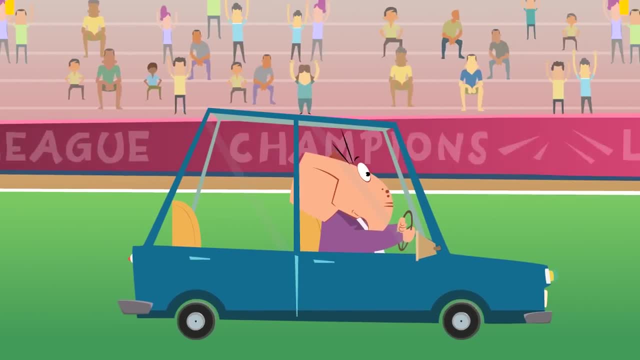 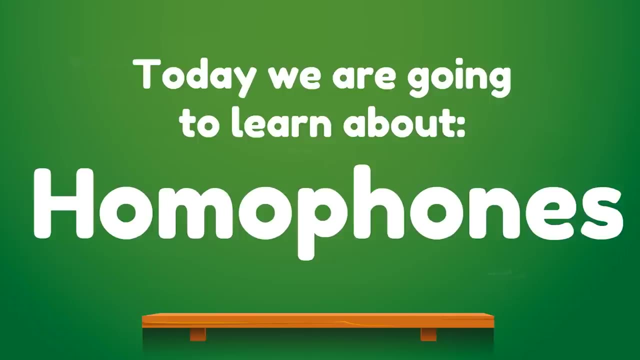 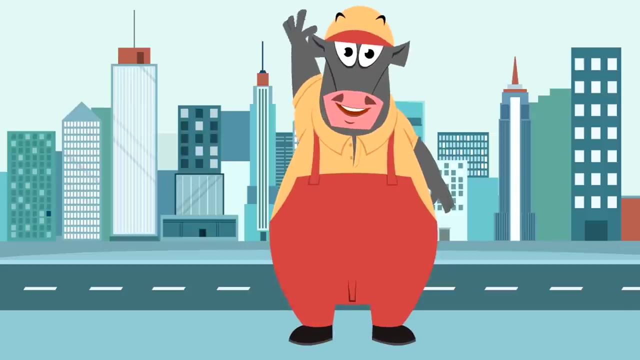 Oh, my goodness, All right. Next we are going to learn about homophones. Homophones are really really weird. okay, They're very weird. Homophones are weird like a cow that works in a city. It just doesn't happen. 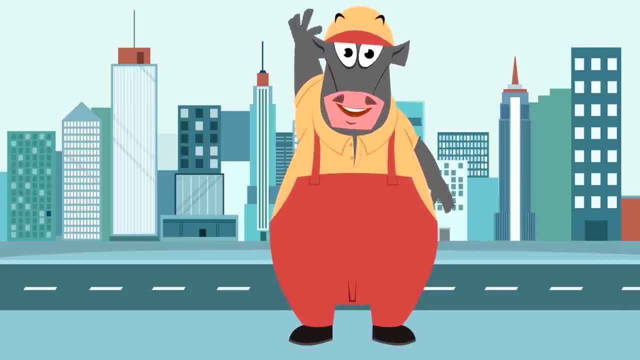 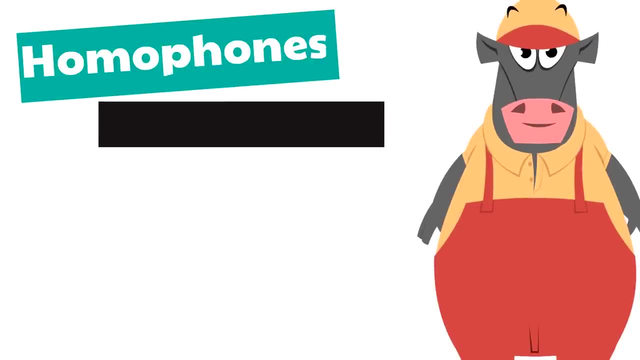 I mean, it's just like what? So many questions? Why is this cow here? Who taught this cow how to wave? Why is this cow wearing clothes? Weird, I don't know if you believe me. Really, homophones are weird. 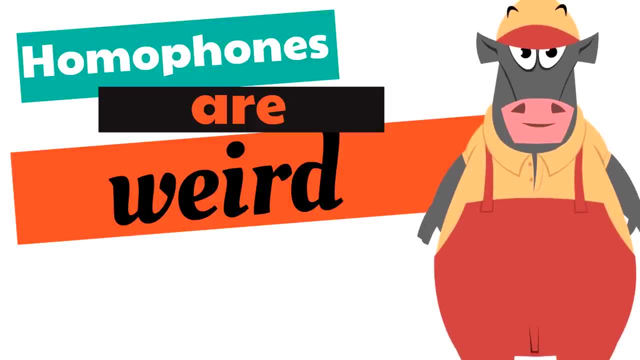 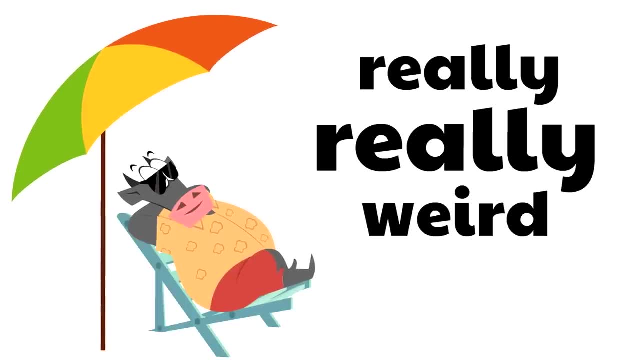 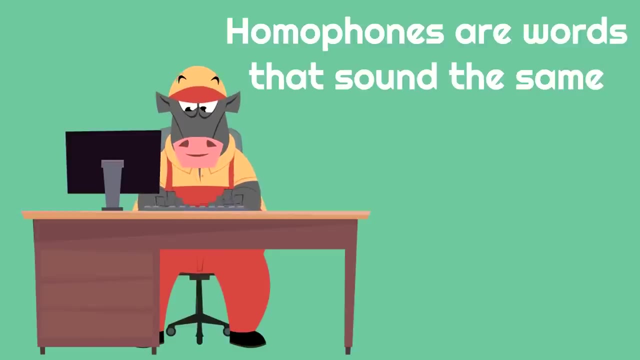 I mean they are weird. I mean really really weird. Okay, I know I'm repeating myself. You need to understand. these are really weird words and we're going to show you why. You see, homophones are words that sound the same but have different meanings and spelling. 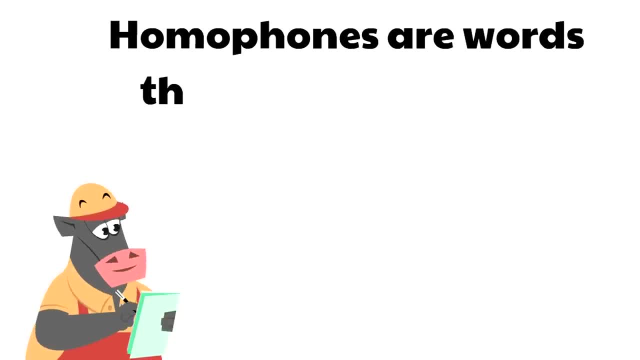 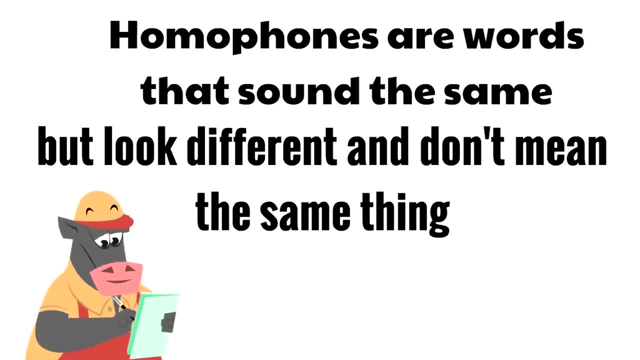 Another way of saying that is: homophones are words that sound the same but look different and don't mean the same thing. They're kind of tricky, weird words that they sound the same but they look different and they don't mean the same thing. 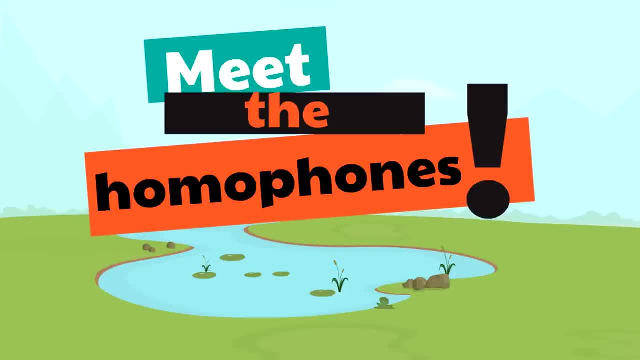 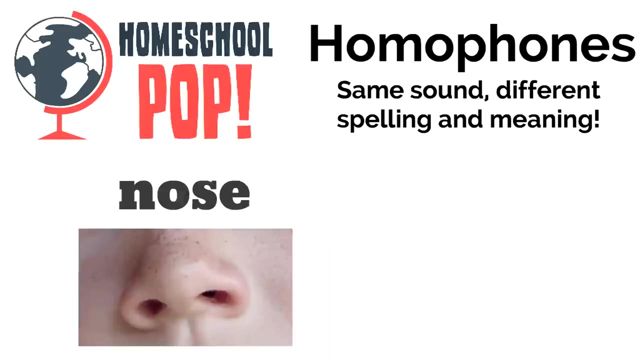 Okay, I think you're ready. It's time to meet the homophones. We want to give you some examples of these words that sound the same but they look different and they don't mean the same thing. Homophones: same sound, different spelling and meaning, like nose and nose. 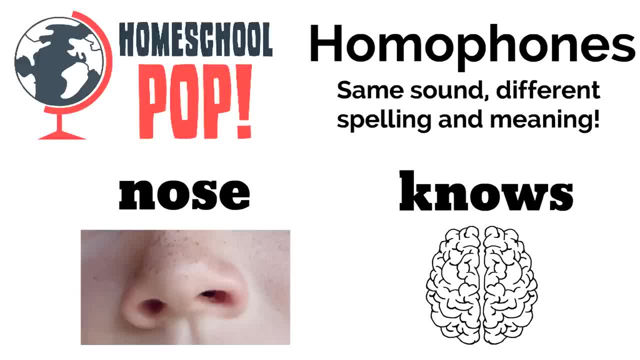 They sound the same, don't they The exact same. They're homophones because they've got very different meanings, don't they? The first nose is a part of your body. The second nose is a part of your body. The second nose is when you have knowledge about something, something in your mind. 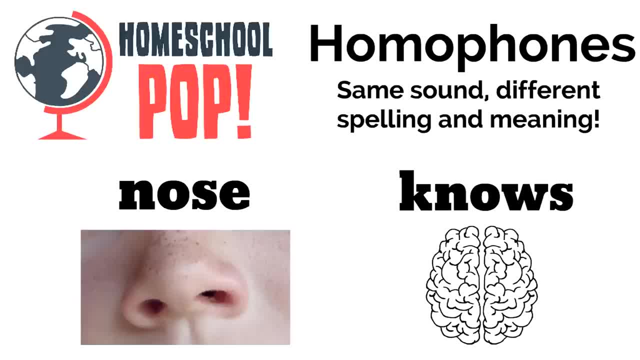 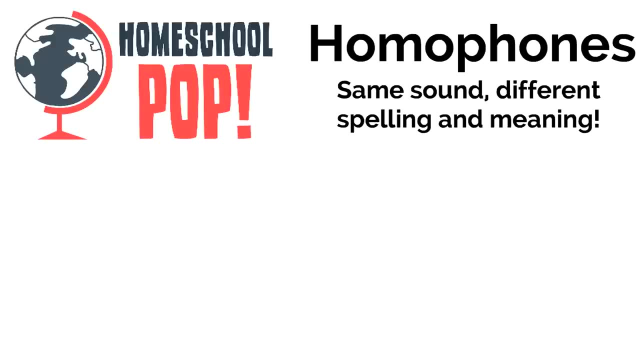 He knows what homophones are. They have the same sound but different spelling and different meaning. It's tricky, isn't it? It's a little weird: Homophones, Homophones- same sound, different spelling and meaning, like eight and eight. 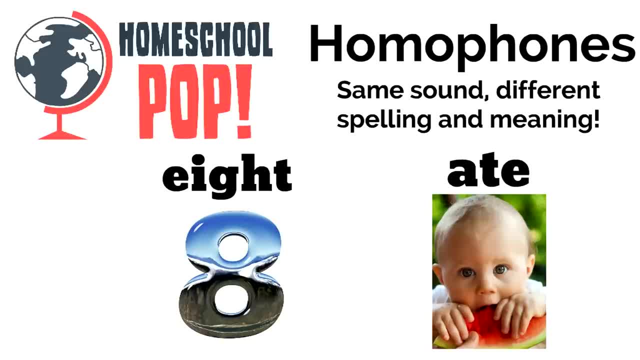 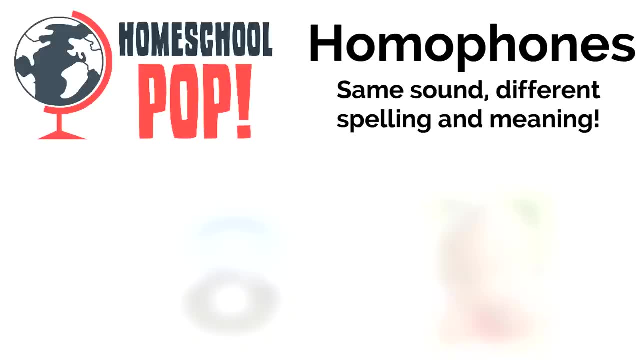 They sound the exact same, don't they? But one is a number right. This first eight is a number. The second eight has to do with eating The baby: ate the watermelon. Eight and eight are homophones. Homophones: same sound, different spelling and meaning, like hay and hay. 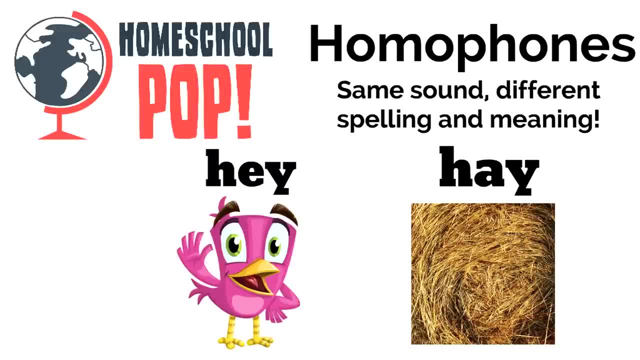 They sound the exact same, but they're homophones, aren't they? Because the first hay means hello and it's spelled differently: Hello hay. It's an informal way of saying hello, just like this friendly little bird is doing right now. 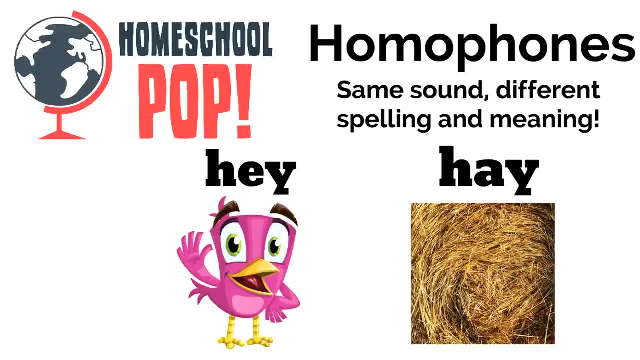 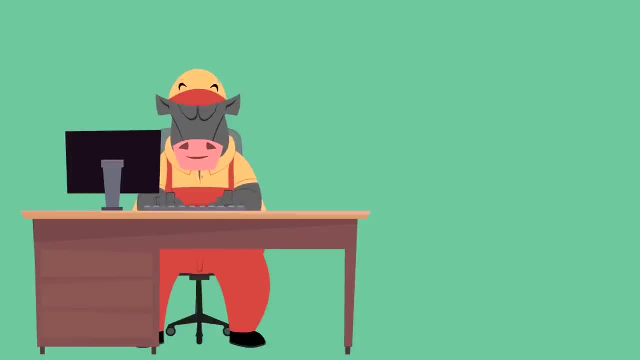 Hey, The second hay is food for horses. They sound the same but they have different spelling and different meaning. Hay and hay are homophones. We want to make sure you really understand this. Homophones are words that sound the same. 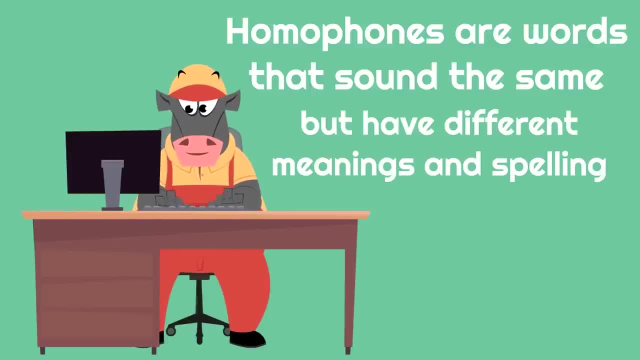 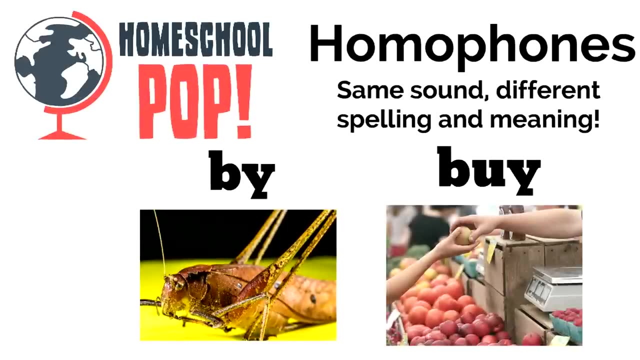 They don't sound the same but have different meanings and spelling, like buy and buy. This first buy means near or close to The photographer that took this picture was by the grasshopper. This second buy means to purchase. You do this at stores, don't you? 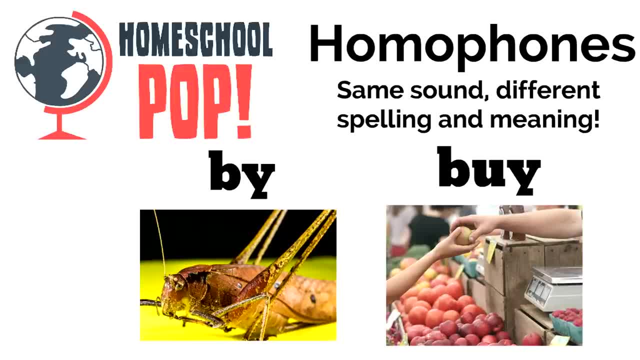 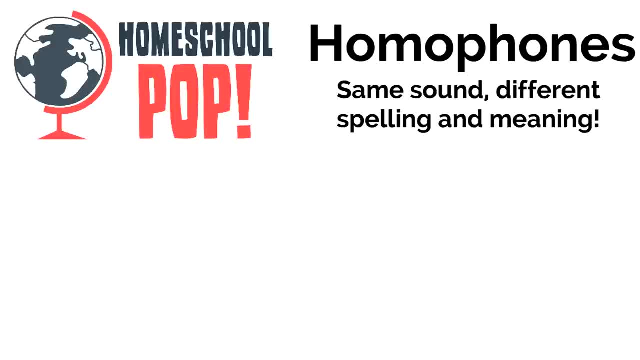 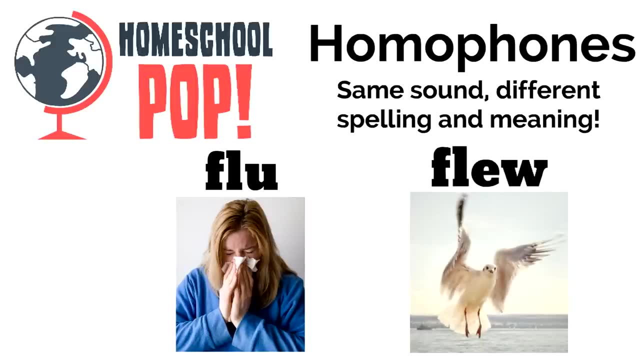 This person is buying an apple, Buy and buy. They're homophones. Here's our final example of homophones: Flew and flew. This first flew isn't very fun at all. It's a type of sickness. The second flew is a lot more fun. 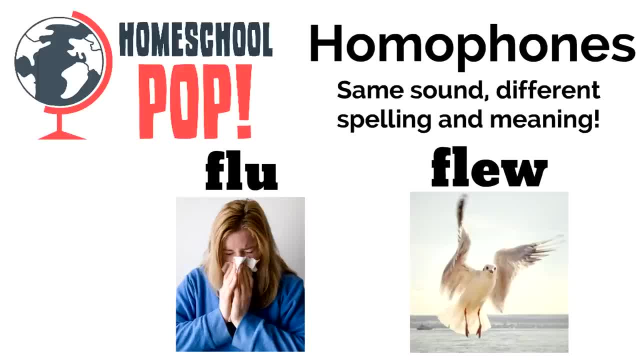 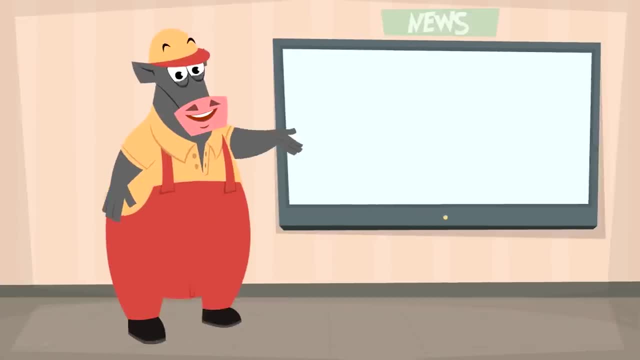 This is a seagull that is flying. The seagull flew over the ocean, Flew and flew. They sound the exact same, but they are very different words, aren't they? They are homophones. Now, this is something crazy. 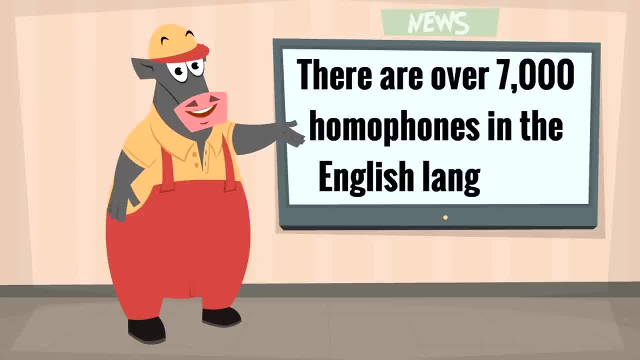 Did you know there are over 7,000 homophones in the English language? Over 7,000!. And that's why we can't talk about all of them here. There are homophones that you probably know, that we didn't have time to cover today. 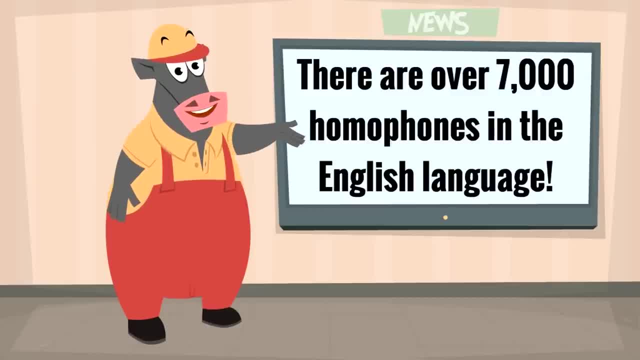 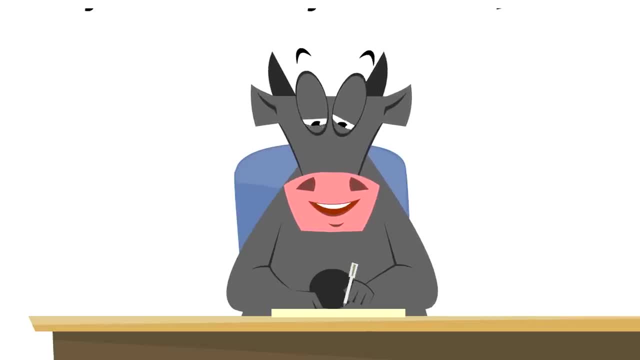 But there are over 7,000 of them in the English language. Hey, Hey, can you think of any other homophones? Maybe, after you watch this video, try to come up with a list of homophones that you might know that we didn't cover in this video. 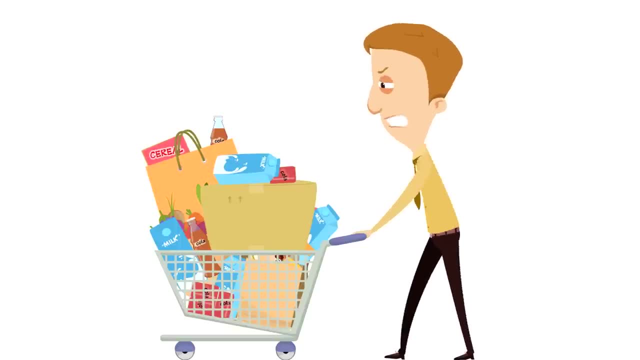 They're a lot of fun. Oh, this is such a heavy cart. Oh my goodness, It's hard work. You know, a lot of times learning can be hard work too, But we hope that these videos are really helpful, Make learning fun, so that learning isn't hard like pushing this cart. 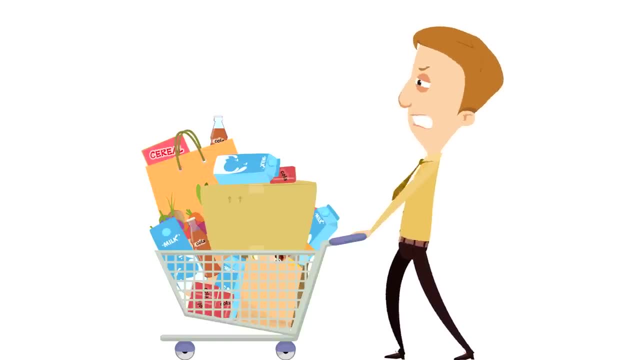 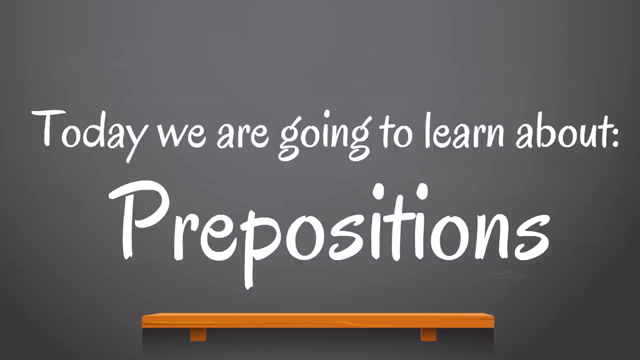 Oh, my goodness. Alright, What's the next thing we should learn about? Let's learn about Prepositions. Yeah, Wow, What a cool sounding word. What are prepositions? You're about to find out, and then you'll just be able to say prepositions. 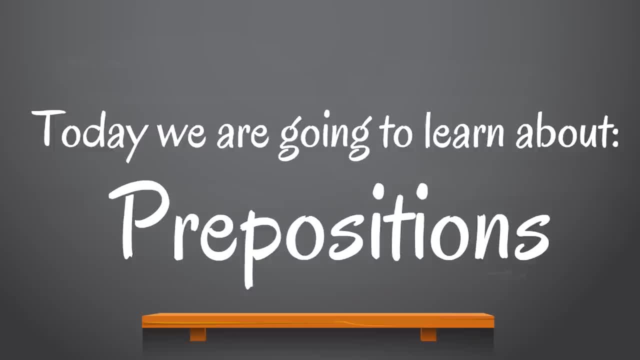 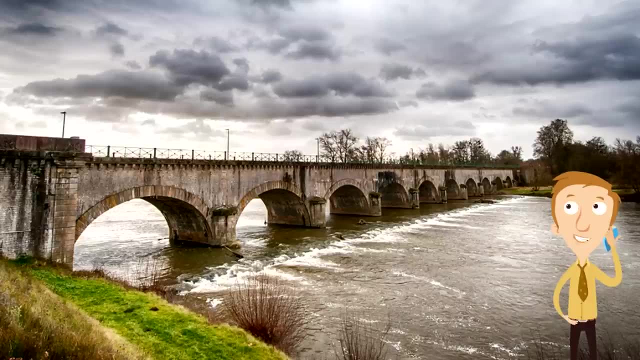 And you'll know exactly what you're talking about. It's going to be cool. First, we want to show you this. Okay, You might be saying: why are you showing us a bridge? Oh, there's a good reason for that. 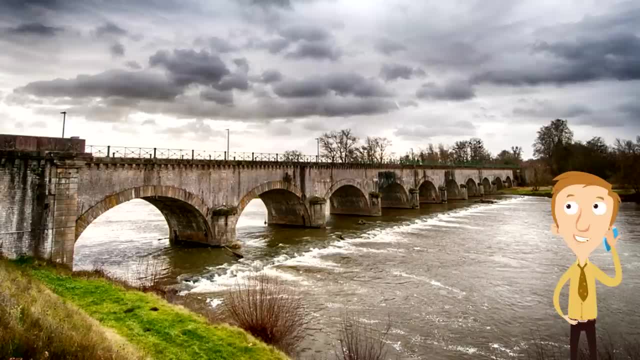 There's a very good reason for that. We're going to just keep that a secret for now. But for now, just look at this picture of a bridge. Bridges are so cool, aren't they? They're so cool. They're structures that connect two sides of things, don't they? 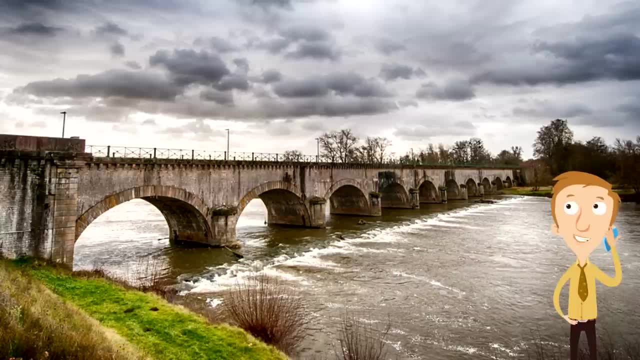 And you can see the storm clouds are coming. It's probably going to start raining. You know the photographer probably was running for cover. You know It's a nice picture of a bridge. Here's another picture of a bridge. Do you know the name of this bridge? 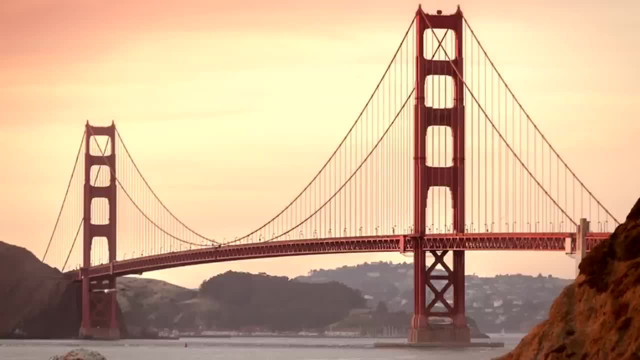 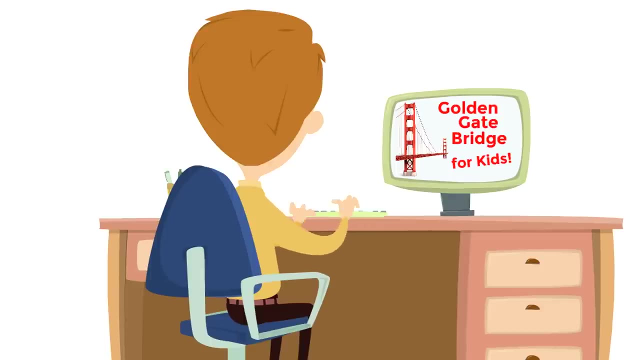 Pretty famous, Pretty famous bridge. Okay, Yeah, The Golden Gate Bridge. Okay, The Golden Gate Bridge. If you didn't know that, you need to check out our video on the Golden Gate Bridge. Some fascinating facts there. You're going to love it. 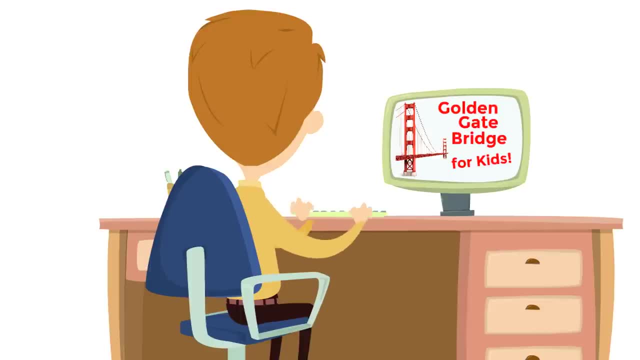 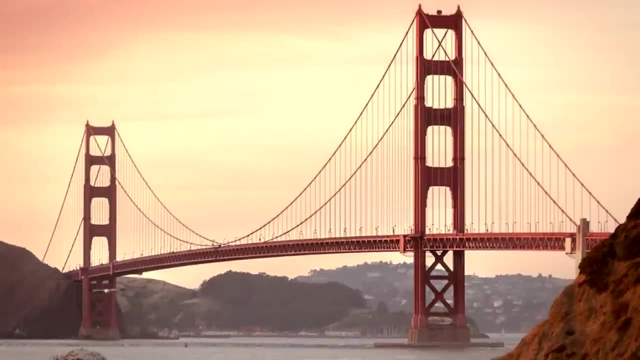 You're going to love sharing those with your friends and your family, And everyone's going to be like what? Let's look at the Golden Gate Bridge again. It's an amazing bridge, And a bridge connects two sides- A bridge. You might be wondering. what does this have to do with prepositions? 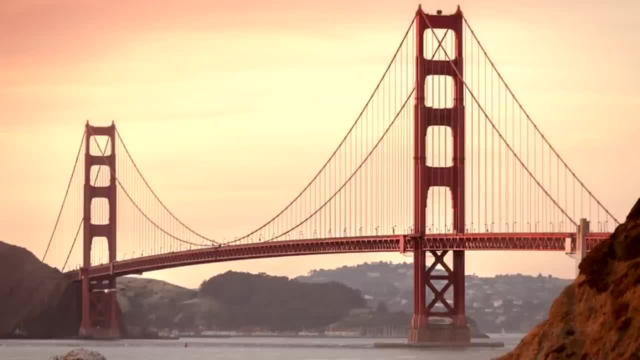 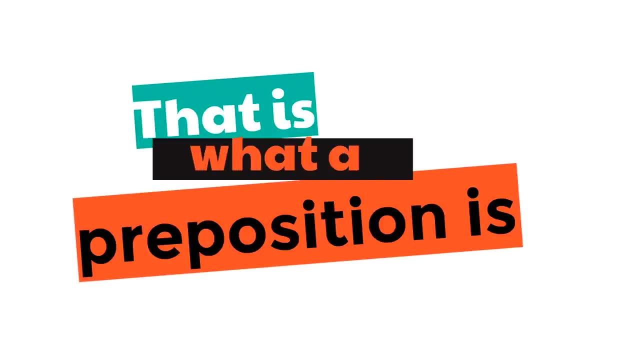 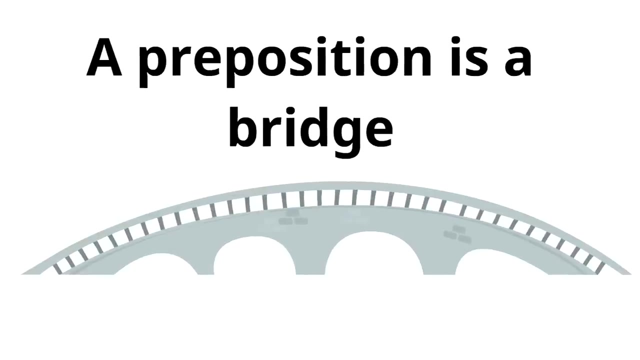 I thought we were talking about prepositions, not bridges. What is going on here? Well, that is what. a preposition is Okay, A bridge. A preposition is a bridge. Okay, In the world of words and grammar, it's not really a bridge. 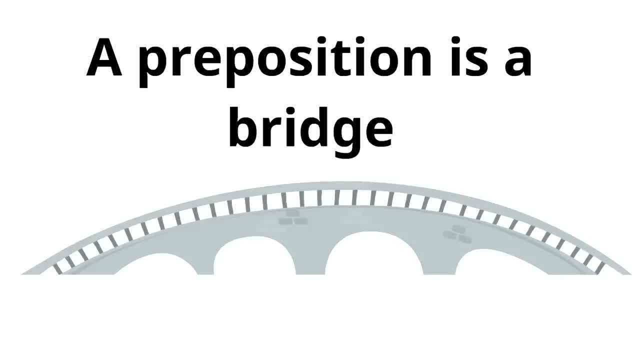 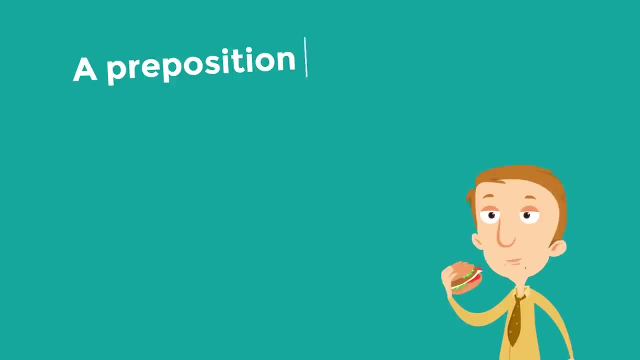 You can't drive a car on a preposition. Okay, That would be a little bit difficult And you wouldn't be able to do it. But a preposition works just like a bridge in the world of words. A preposition is a bridge that comes before a noun or pronoun. 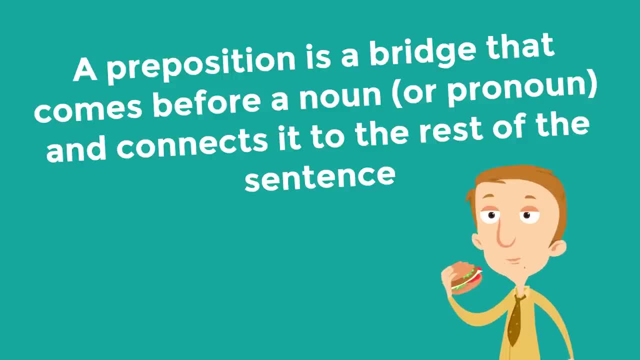 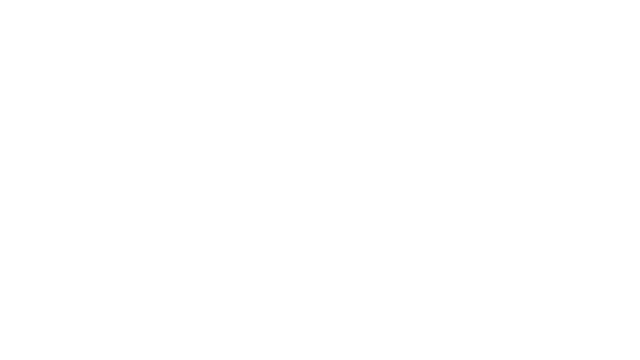 Okay, And connects it to the rest of the sentence, And this is how it works. For example, let's say we've got a noun at the end here, And then we've got the rest of the sentence. Now we've got a problem. 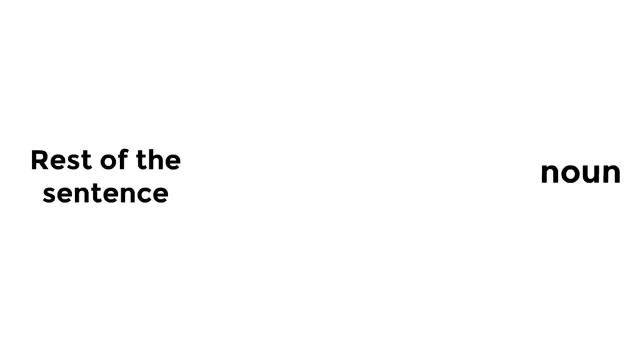 There's a big gap, Something's got to go in between. Now, let's say the part with the noun is my backpack And the rest of the sentence is: I put my book. I put my book, My backpack. There's a gap. 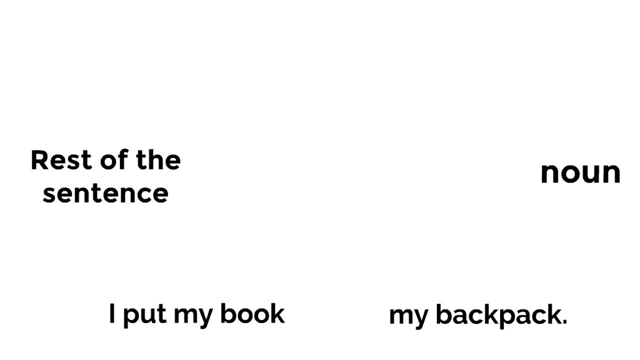 I mean, it's a lonely backpack. We need a connecting word, We need a bridge. So we put in a preposition- Yeah, A preposition, A bridge word, A connecting word that will connect the noun at the end to the rest of the sentence. 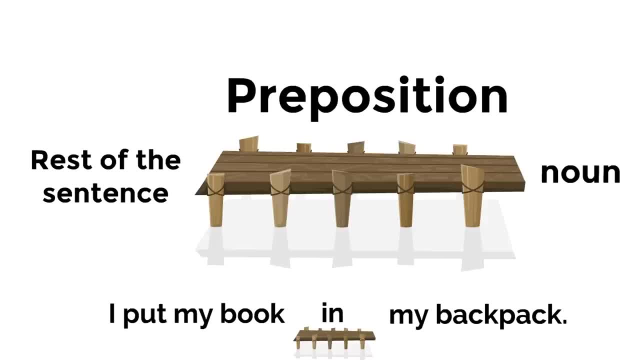 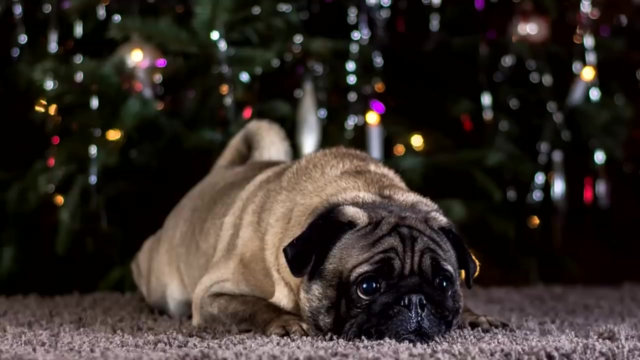 So we're going to use the preposition in. So it would read like this: I put my book in my backpack. Now the noun backpack is connected to the rest of the sentence. Yay, Yay, bridge, Yay prepositions. 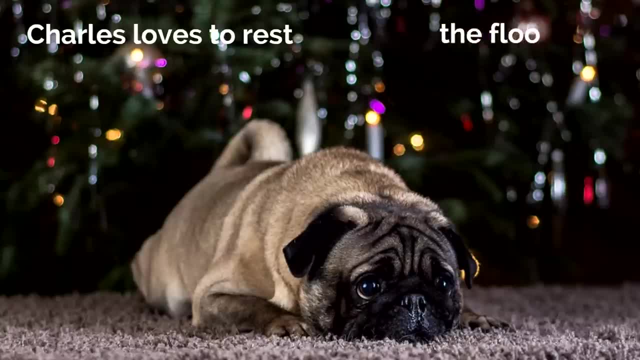 Let's look at this example. Charles loves to rest The floor. Uh-oh, There's a gap. We're going to need a bridge, We're going to need a preposition to connect floor to the rest of the sentence, aren't we? 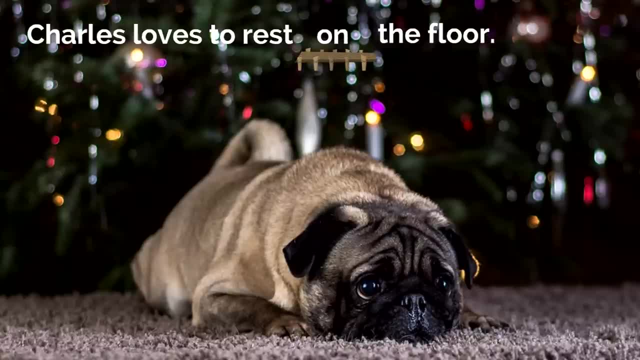 Let's try the preposition on: Charles loves to rest on the floor- Oh, it's perfect. On is connecting floor to the rest of the sentence. Charles loves to rest on the floor- Oh, it's perfect, That's perfect. 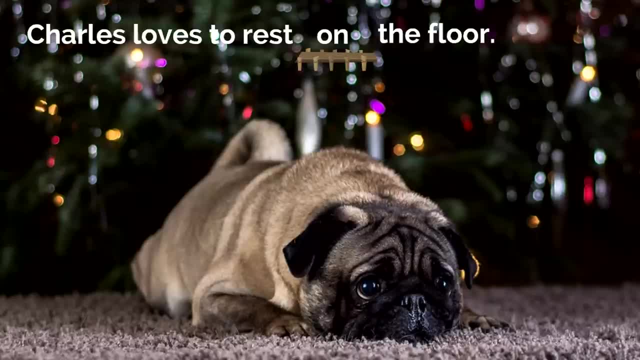 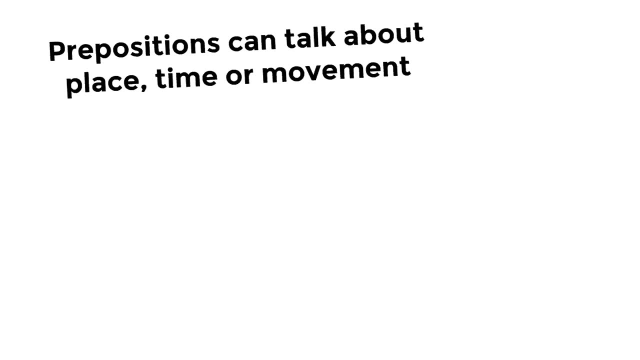 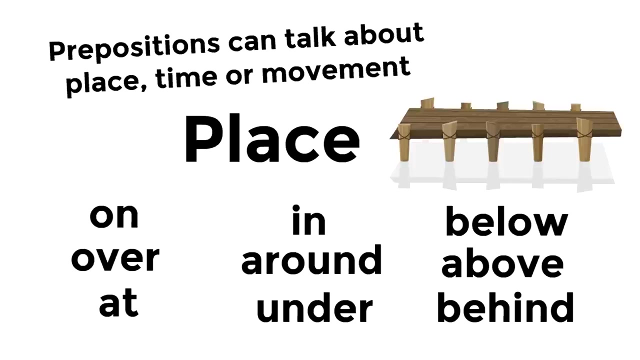 I love prepositions. Prepositions can talk about place, time or movement. Here's some examples of prepositions that talk about place: On, over, at, in, around, under, below, above, behind. These are all prepositions that talk about place. 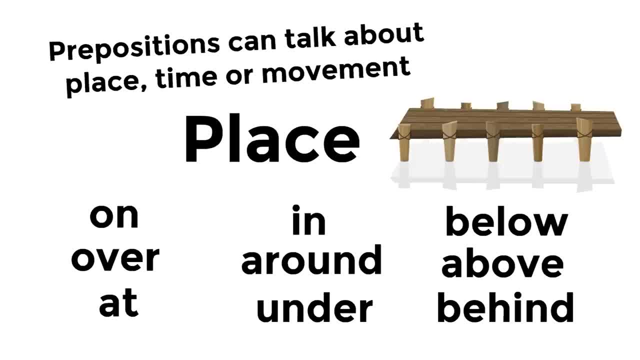 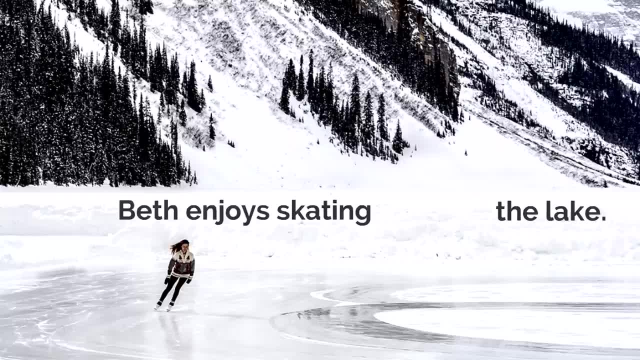 Isn't that interesting? Let's look at this example. Beth enjoys skating the lake. Uh-oh, There's a gap. We need a preposition. We're going to need a preposition that talks about place. Let's try around. 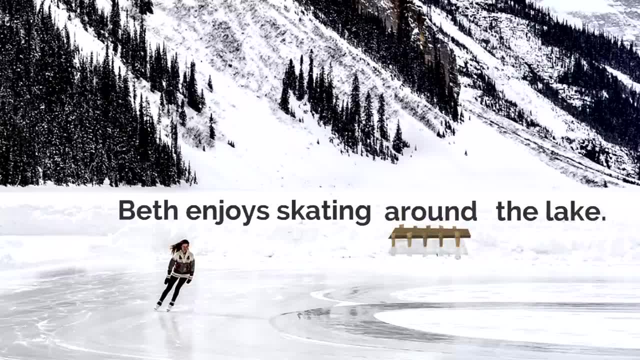 Beth enjoys skating around the lake. Oh, that's the perfect preposition for that. It connects lake to the rest of the sentence. To the rest of the sentence: Beth enjoys skating around the lake Prepositions: We said this already. They're pretty cool. 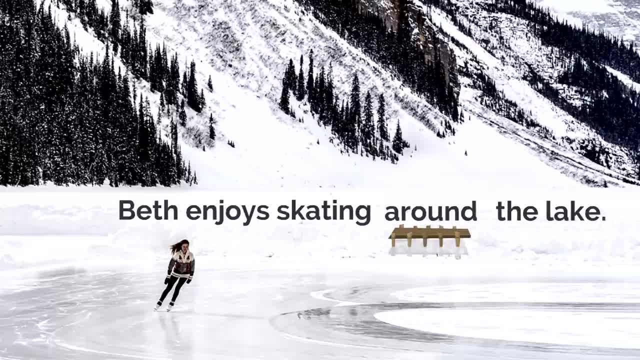 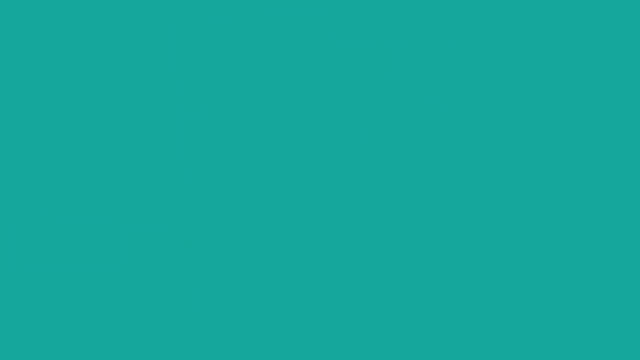 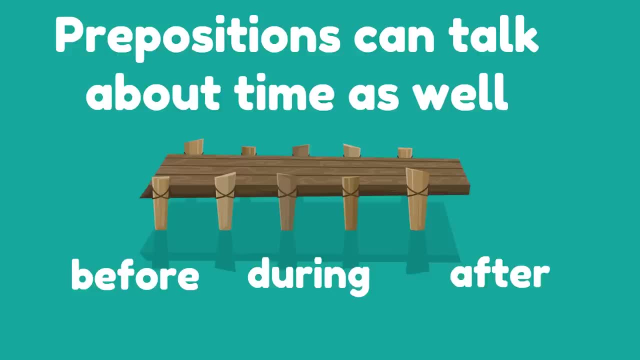 They're pretty awesome, Pretty amazing. All right, You got to connect. We need the connecting words, We need the bridges, We need prepositions. Now, prepositions can talk about time as well. Look at these prepositions: Before, during, after. 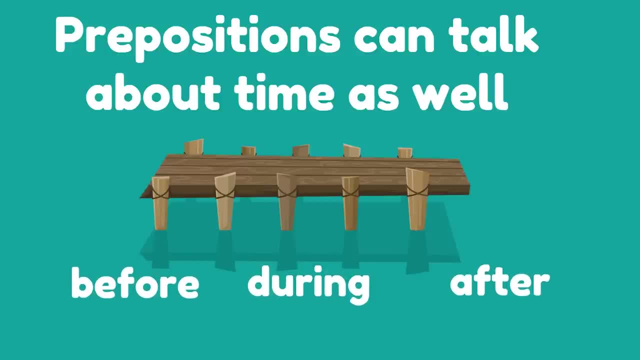 These are prepositions. These are bridge words, Connecting words. They're prepositions that talk about time. Look at this example: It snowed four inches the day. Oh, we're definitely going to need a preposition there, aren't we? 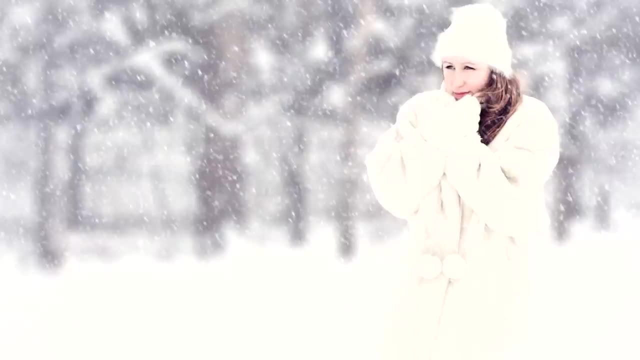 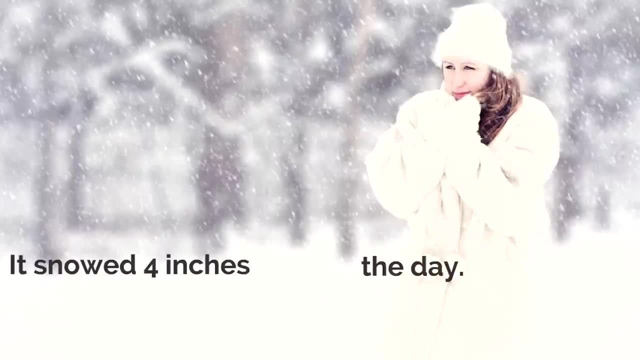 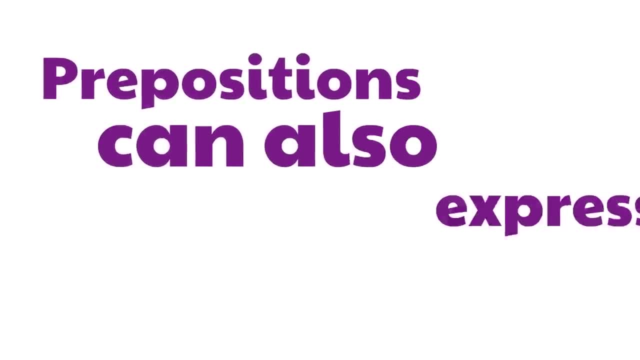 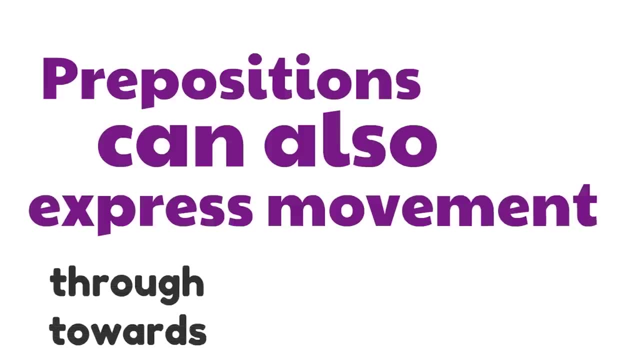 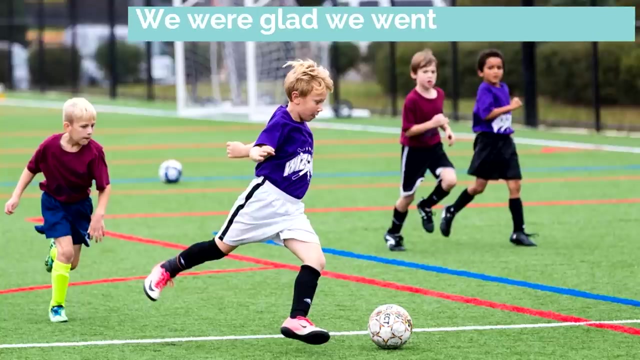 Now, prepositions can also express movement. Whoa, Like these prepositions: Through, towards, to, into, across, along. These are prepositions, bridge words, words that express movement. let's try this one. we were glad we went the game. 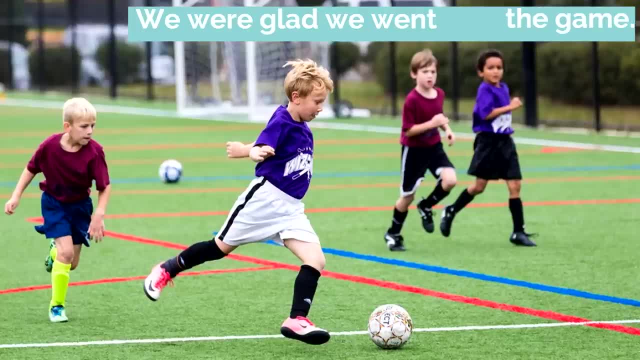 uh-oh, we're definitely gonna need a preposition. we have to connect game to the rest of the sentence. let's try to. we were glad we went to the game to is one of the prepositions that express movement. we were glad we went to the. 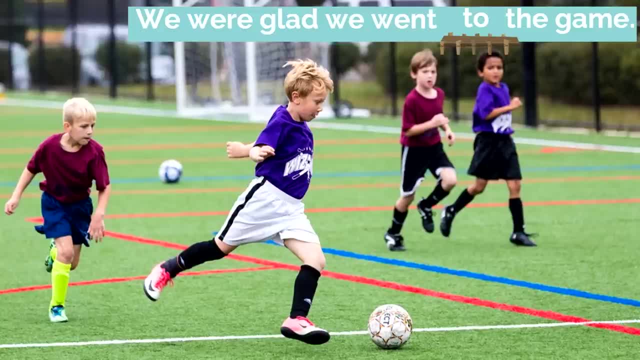 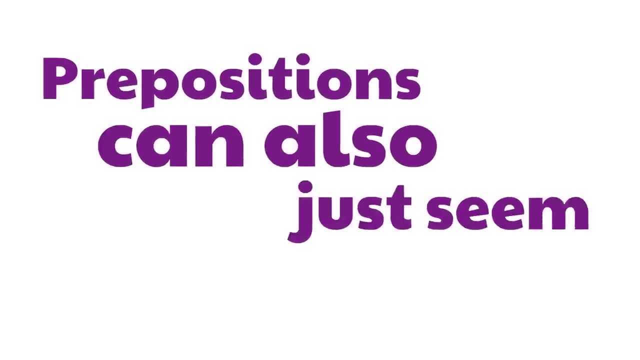 game, and now the word game is connected to the rest of the sentence. prepositions can also just seem random, like about, of and from. you could just memorize these words as prepositions, because they do kind of seem random about of and from. you could just memorize these words as prepositions because they do kind of seem. 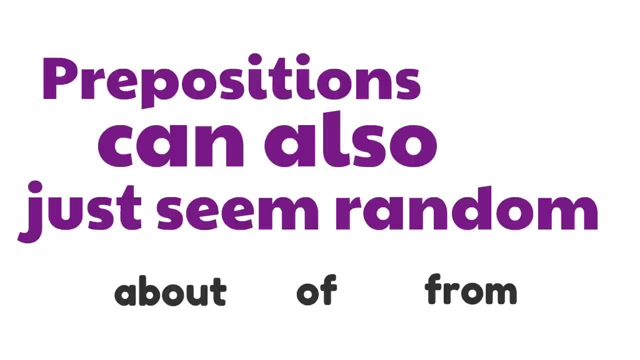 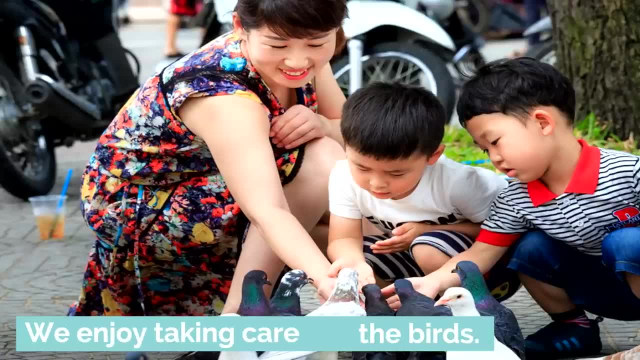 from are all prepositions too. here's our next sentence. we enjoy taking care the birds. uh-oh, there's a gap. we're gonna need to fill that with a bridge word, a preposition, aren't we? what is a preposition that you think would go well there? which one do you think fits in? 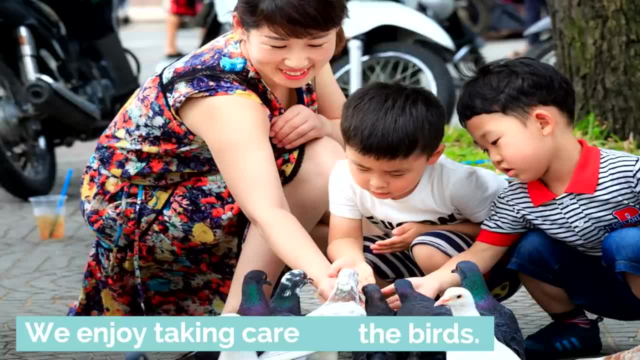 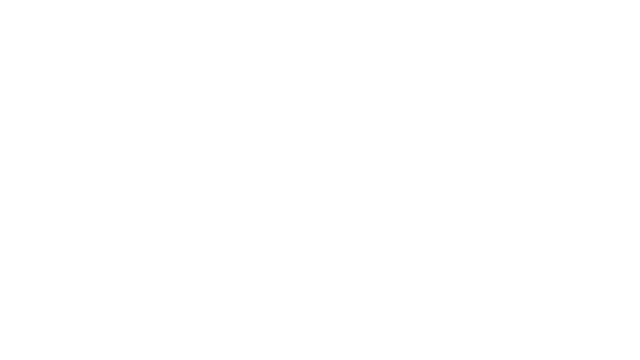 that like a puzzle. we enjoy taking care the birds, yeah of of. we enjoy taking care of the birds of is a preposition. it's a bridge word connecting birds with the rest of the sentence. now here's something that can be tricky. prepositions can also appear at the. 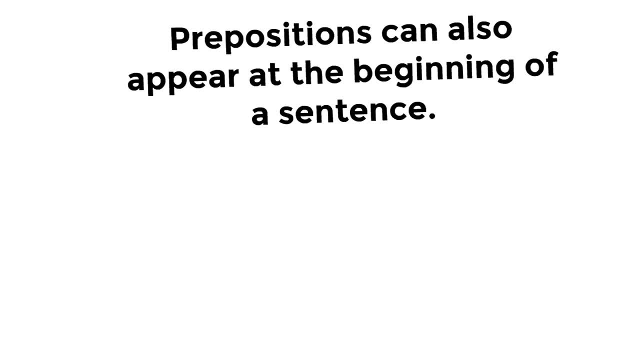 beginning of a sentence, the preposition still has a noun coming after it, and then there's the rest of the sentence, but the preposition is still connecting the noun to the rest of the sentence. let's show you with an example. all right, here we go after dinner. after is the preposition: after dinner. 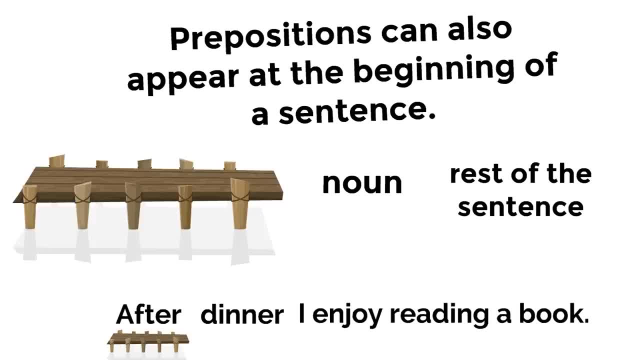 I enjoy reading a book. Wow, now notice it's still a bridge word and it's still connecting dinner. that's the noun to the rest of the sentence. even though it appears at the beginning, it's still a bridge word, still a connecting word. so if you see a preposition at the beginning of a sentence, don't freak out. 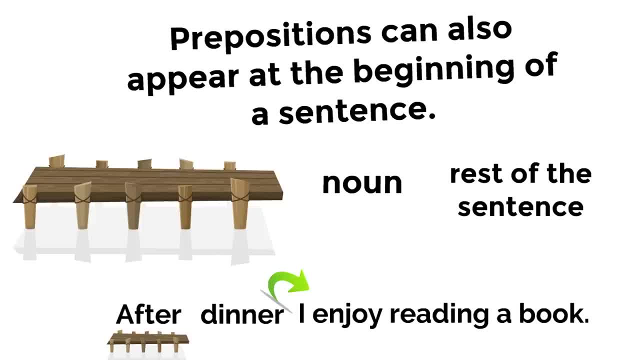 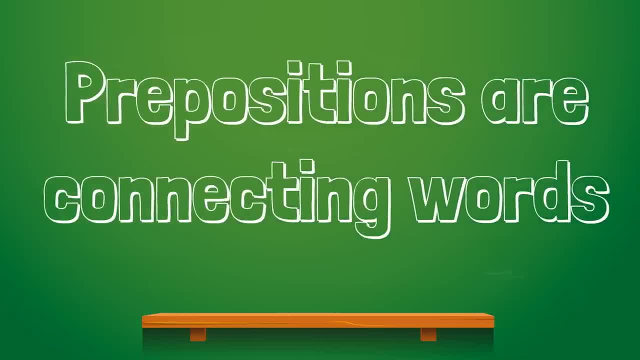 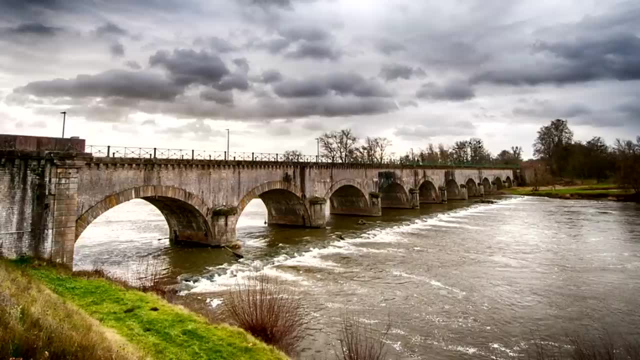 it's okay. sometimes they go there, prepositions are connecting words and Wow, just like bridges. they're a great time, they're awesome and they just they're just cool. they're just cool. who else is a fan of prepositions? anybody, anybody. no, you like prepositions now, right, you love them. right, you love. 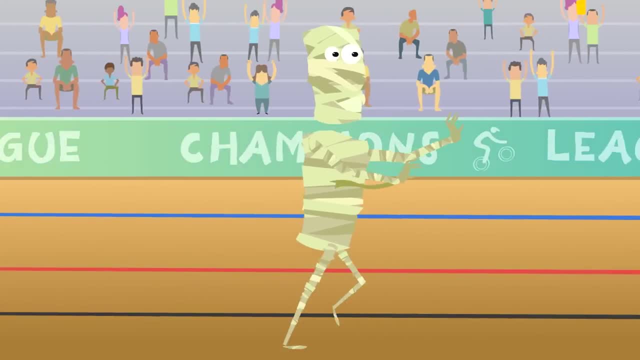 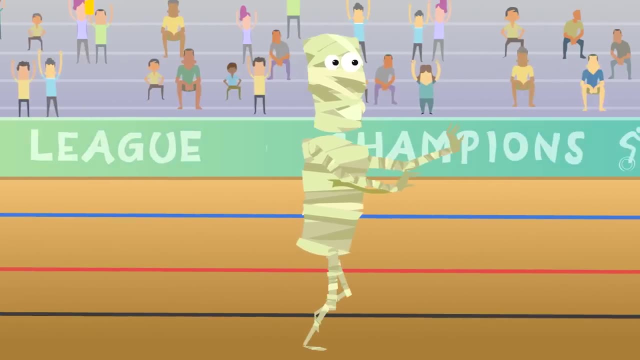 prepositions, they're connecting words, they're bridge words. Wow, mommy, you're doing such a great job in your race. I had no idea you were an athlete. okay, I mean, with all that cloth wrapped around, you're doing great. you're doing a great job, just like these kids are doing a great job. 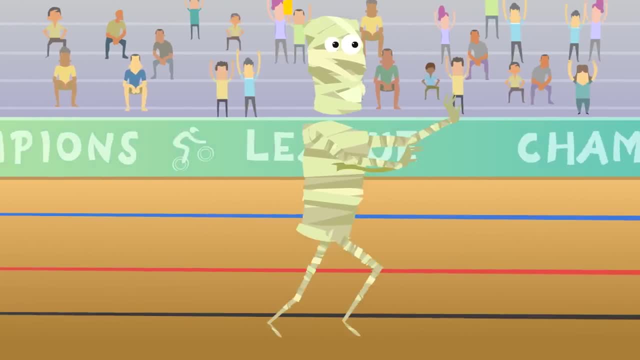 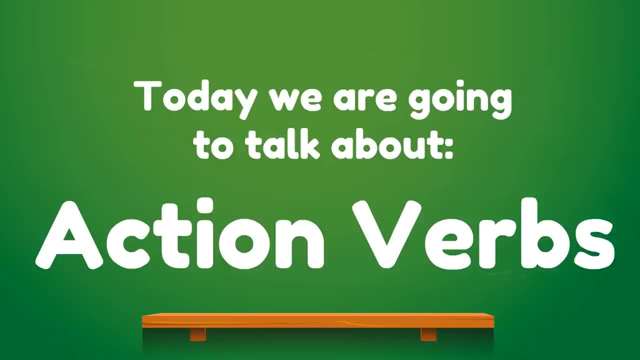 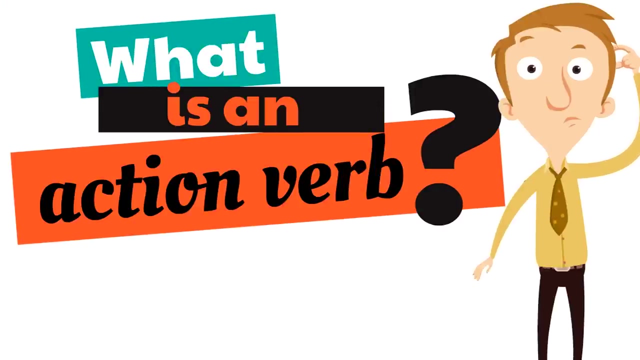 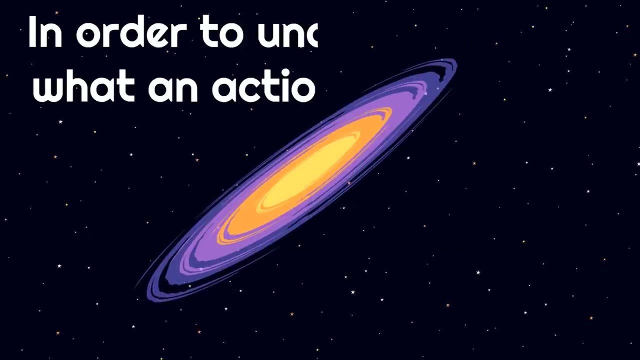 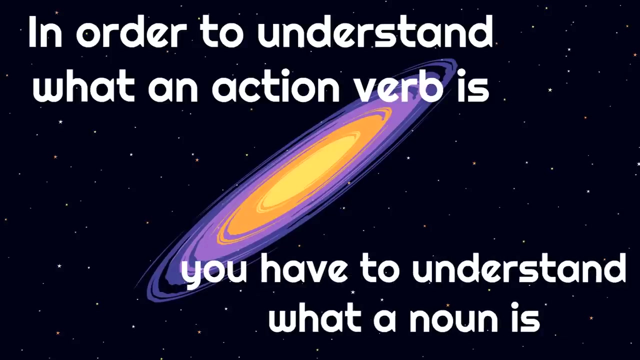 learning. in fact, how about this? the next thing we're gonna learn about is action verbs, which sounds exciting because it is exciting. well, first things first. what is an action verb? huh, what is an action verb? the truth is, in order to understand what an action verb is, you have to understand what a noun is. remember a. 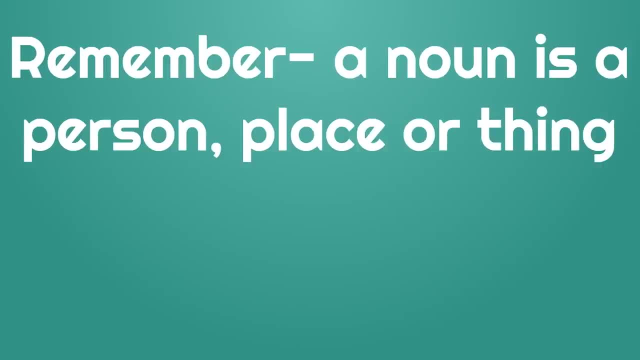 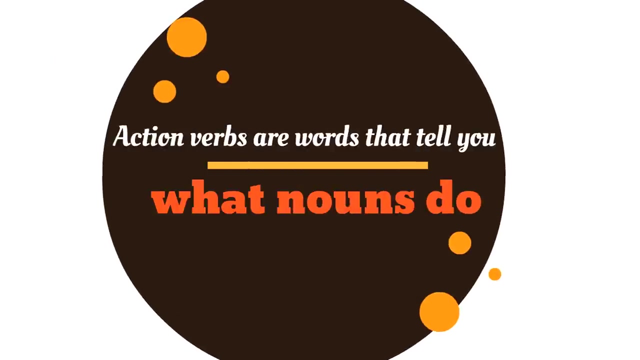 noun is a person, place or thing: a person like a teacher, a place like a gas station or a thing like an alarm clock. if it's a person, place or thing, it's a noun. okay, so what is an action verb? well, action verbs are words that tell you what nouns do. oh, it's so cool, we'll. 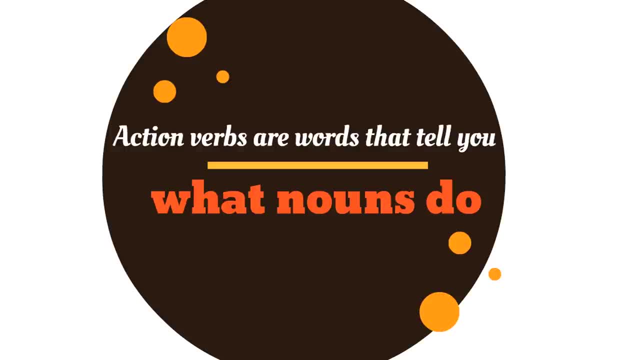 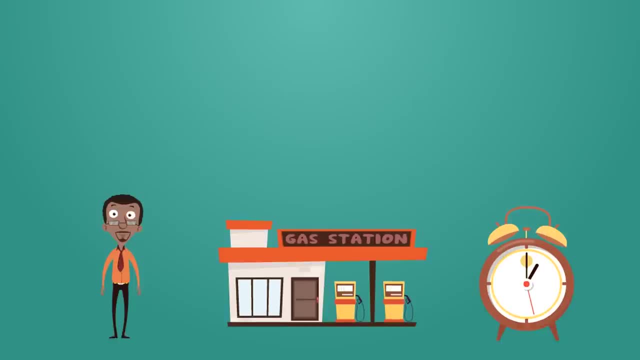 say it again, action verbs are words that tell you what nouns do, and we'll give you some examples. all right, now we're gonna look at some action verbs for the nouns we just saw. remember, action words are words that tell you what nouns do. so our first one: what do teachers do? 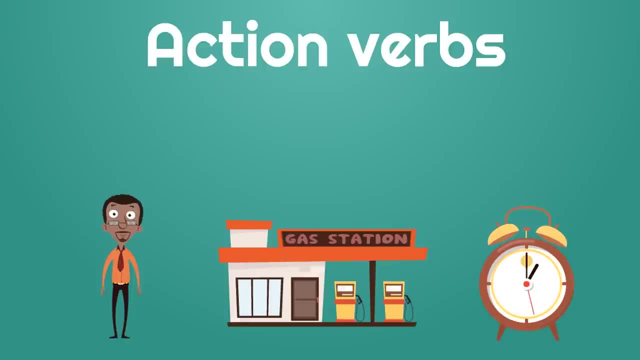 what does this teacher do? yeah, he teaches. teaches is a good action verb. it's what this noun does, what this teacher does. what else does this teacher do? this teacher helps, yeah. all right on to the gas station. what does a gas station do? well, gas station sells, doesn't it it? 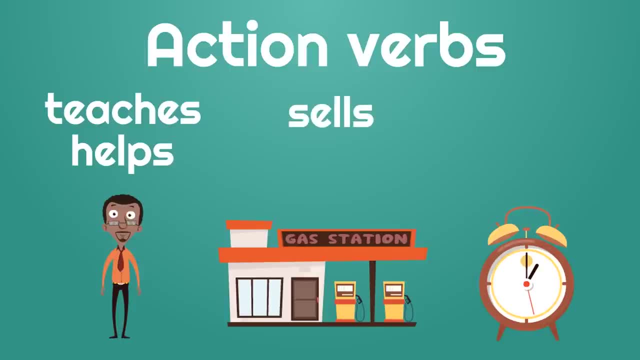 sells gasoline and other things. what else does the gas station do? so, according to the gas station do, What's another action verb for a gas station? Well, gas station fuels. The gas station fuels your car. Fuels is an action verb. Great, Let's try the alarm clock. What does an 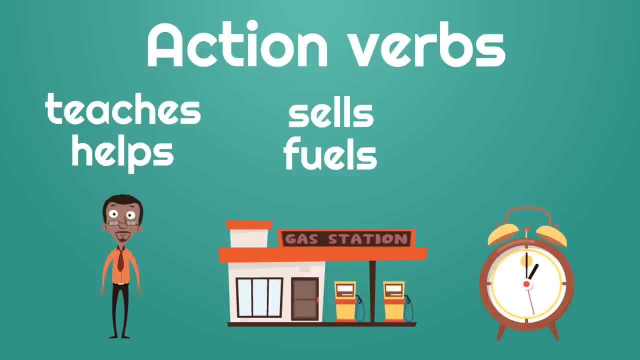 alarm clock do. What are some action verbs that describe what an alarm clock does? Well, an alarm clock ticks, doesn't it? Tick, tick, tick, tick. That's one action verb for an alarm clock. Another action verb: let me give you a hint. This is what an alarm clock does when you need to wake. 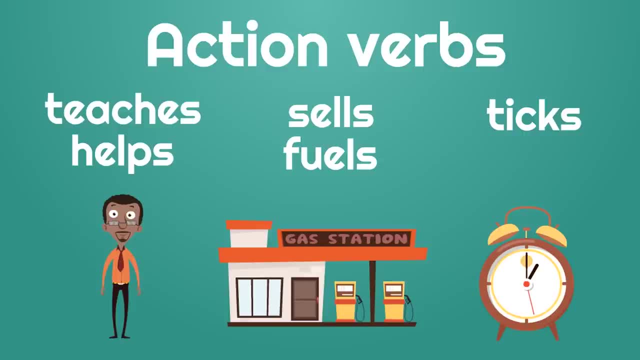 up. What does an alarm clock do when you need to wake up? It rings, Yeah, An action verb is rings. Action verbs describe what nouns do. A teacher teaches and helps, A gas station sells and fuels, And an alarm clock ticks and rings. 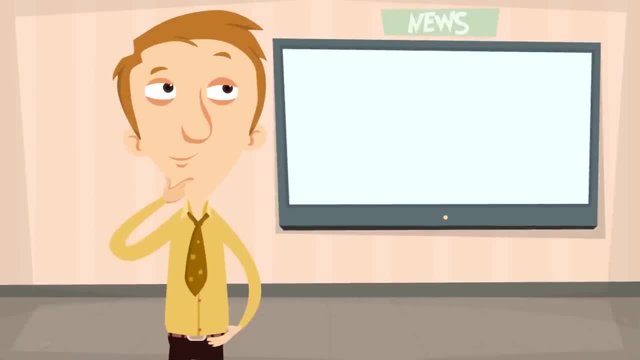 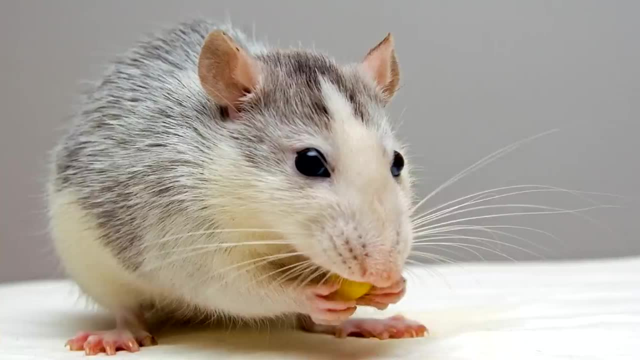 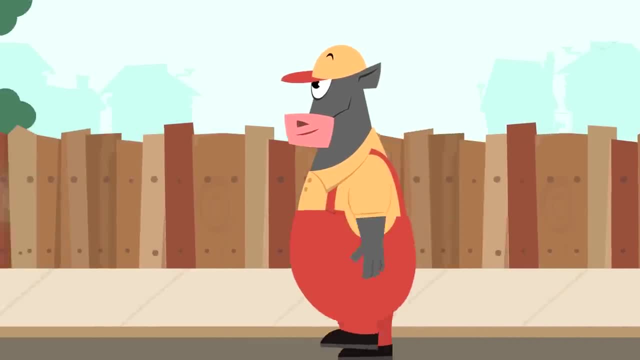 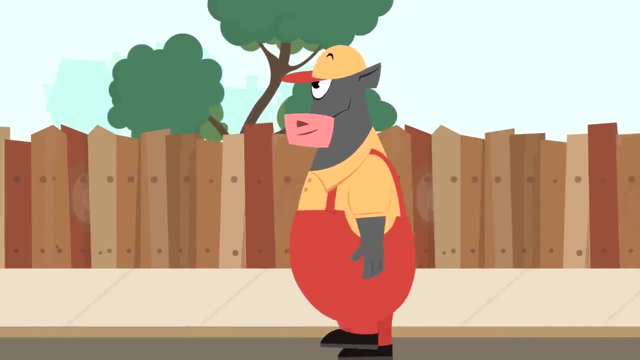 Oh, wow, look, it's the homophone cow. Homophone cow, Homophone cow. You're just walking, you're just going to ignore me. See how it is Okay, so you're upset that we haven't included you in other videos. 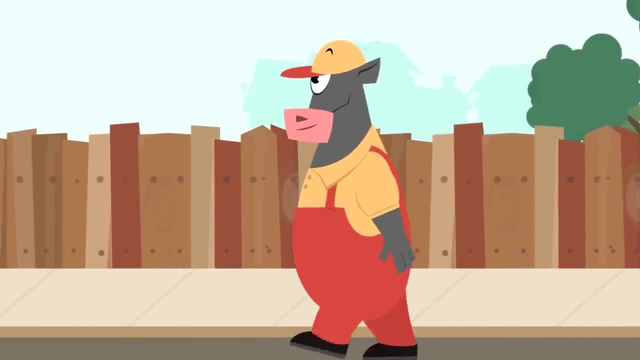 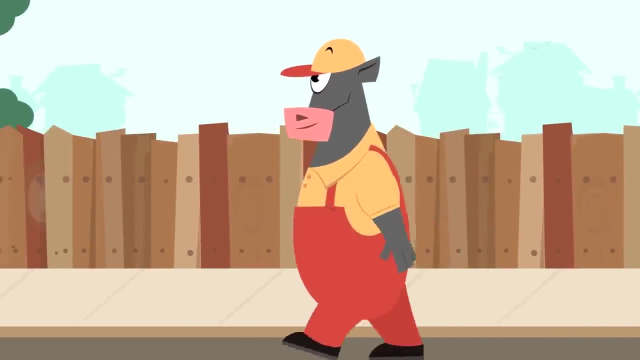 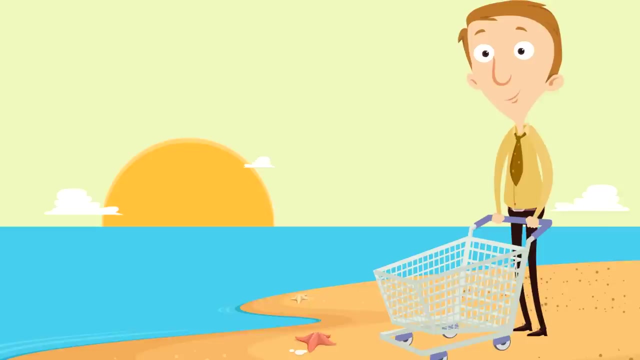 What do you call this? You know you're in a compilation video. That's cool too. All right, I need to talk to the homophone cow, But in the meantime, let's learn about sentence fragments. Ah, the beach is so wonderful, isn't it? 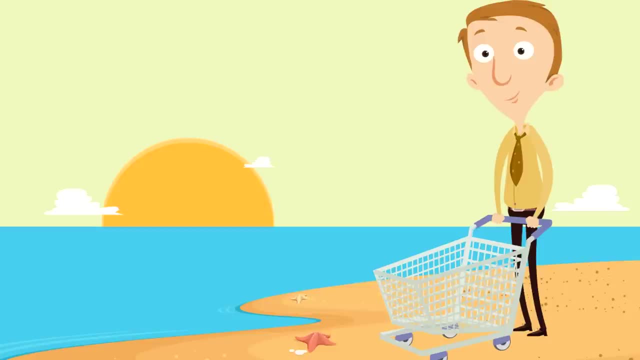 Don't you just love the beach? I'm standing here with my shopping cart and there's one word that comes to mind When I'm standing here looking at the sun setting: this is complete. What else could you want? You're standing on a beach. 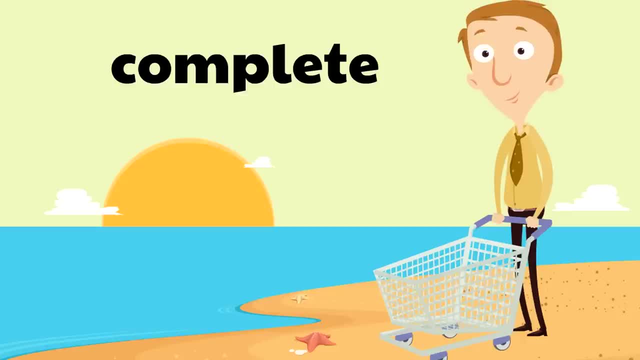 Don't make fun of the shopping cart. I might find something on the beach. okay, You don't bring a shopping cart to the beach. That's weird. okay, I've got a shopping cart. I feel complete. This is complete to me. 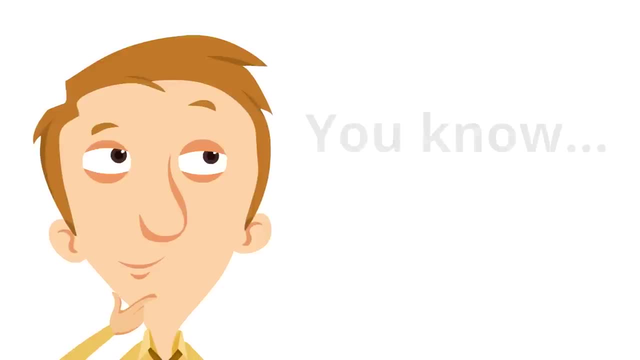 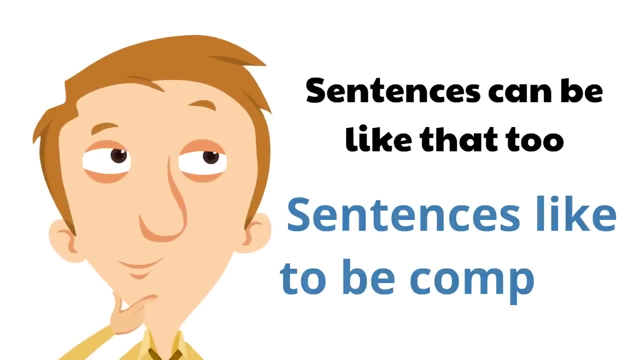 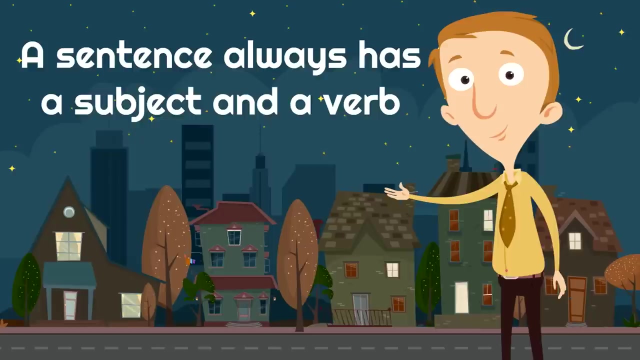 This makes me feel happy. You know, sentences can be like that too. You see, sentences like to be complete. They love to be complete. A sentence always has a subject and a verb. A sentence wants to be complete because without a subject and a verb, it's not a sentence anymore. 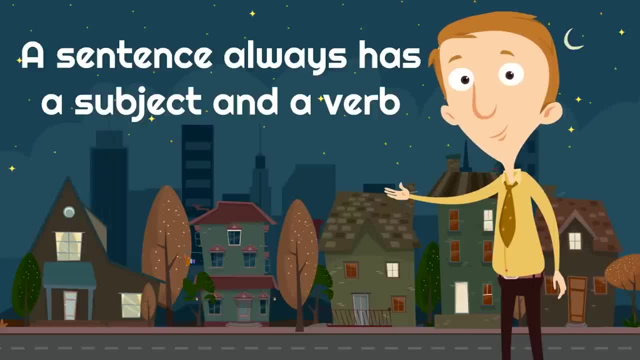 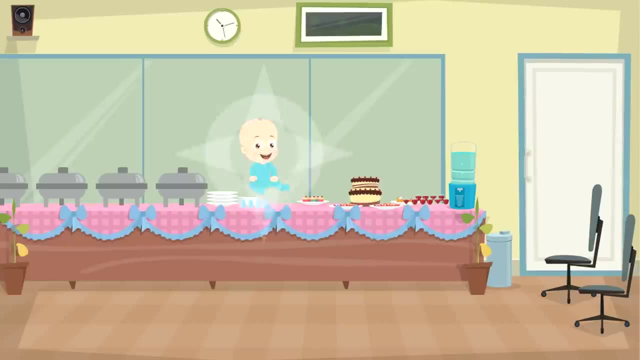 In fact it's something else. It's a sentence. It's fragment, It's fragment, But let me not get too far ahead of myself. Always remember: a sentence must have a subject and a verb, Kind of like every cool birthday party must have a baby and Chomsky. 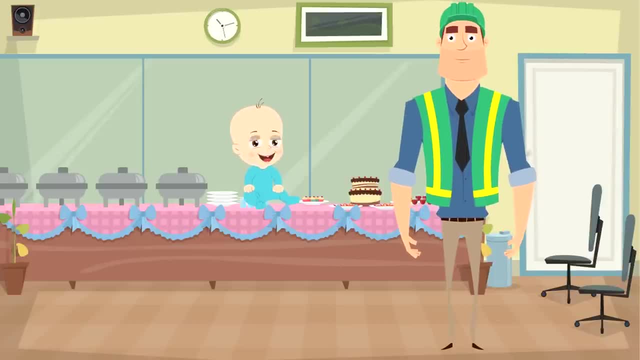 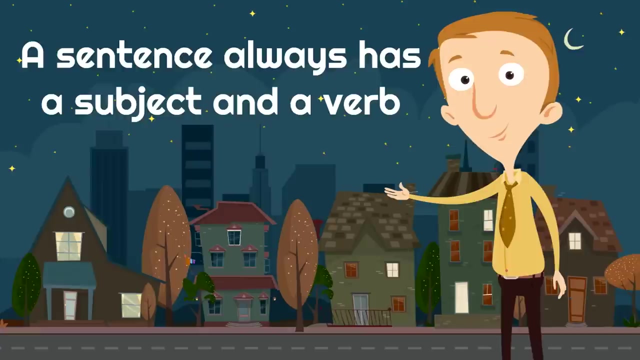 I mean maybe a baby and Chomsky. I haven't forgotten about the hat. I haven't forgotten about the hat. So You can come to my party, but it's still raw, still still hurts, starts. all right, let's get back again. so a sentence always has. 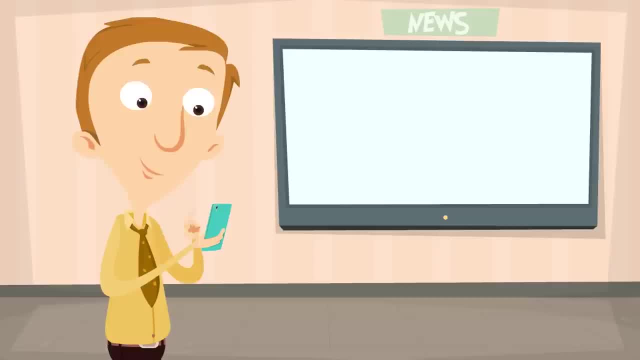 a subject and a verb. that means a sentence is a group of words that has a subject and a verb. it needs to have both, otherwise it's not a sentence. a sentence is a group of words that has a subject and a verb. like this, the dog plays catch. 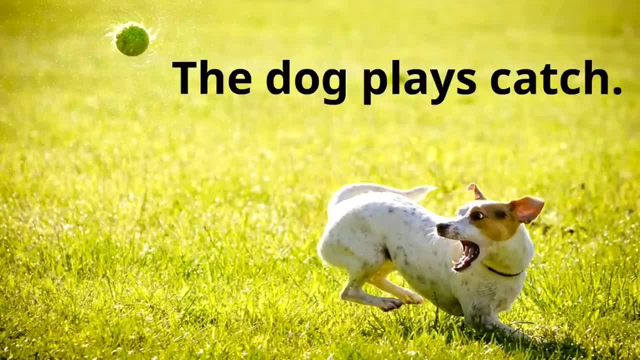 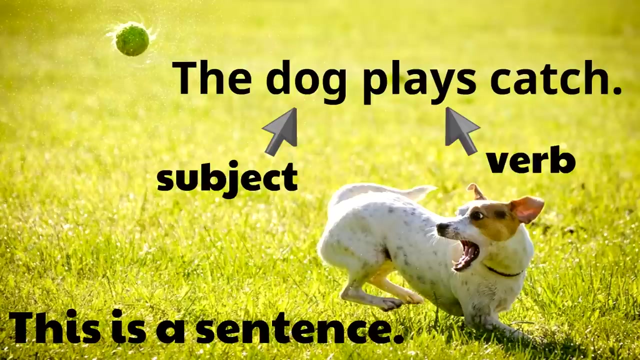 does it have a subject and a verb? yeah, the subject is the word dog and the verb is: which word? which word is the verb? yeah, plays. this is a sentence. it has a subject and a verb, which means it's expressing a complete thought. this is complete. there's a. 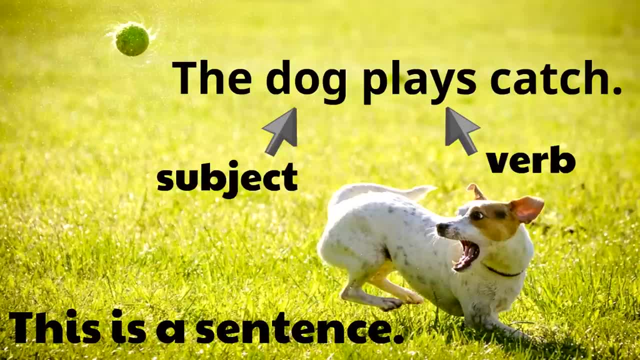 subject: there's a verb, we know what's going on and there's no way this dog is catching this ball. or maybe this dog will catch the ball, who knows? let us know in the comments which one you think will happen. you think he's gonna catch it, or? 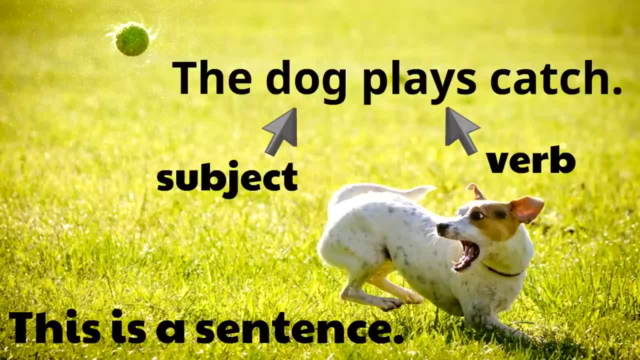 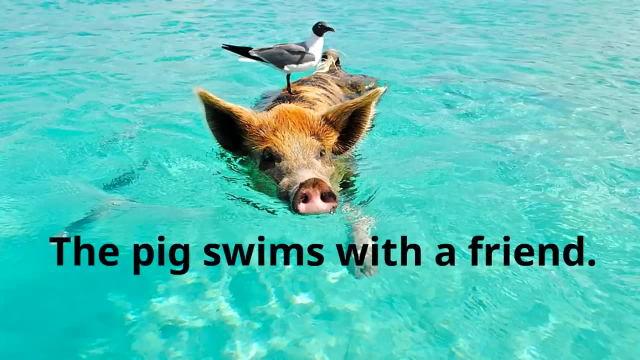 do you think it's gonna fall to the ground? who knows, but this is a sentence. this is complete. it has a subject and a verb. it's a sentence. or look at this one: the pig swims with a friend. the pig swims with a friend. is there a subject and is there a verb as well. well, yeah, the subject is pig, the. 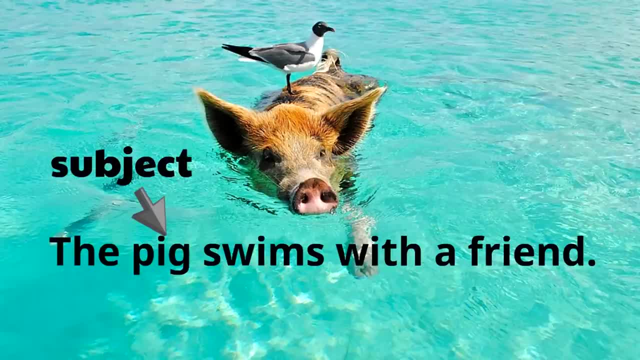 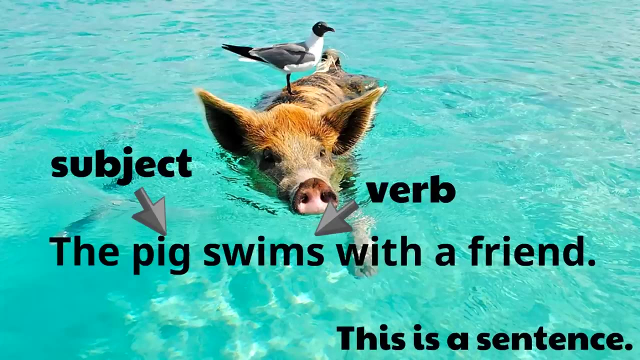 pig, but is there a verb? which word is the verb? yeah, swims. so this has a subject and a verb. this is a sentence. I mean it's got a subject and it's got a verb and it's expressing a complete thought. it's not missing anything, it's complete, it's got. 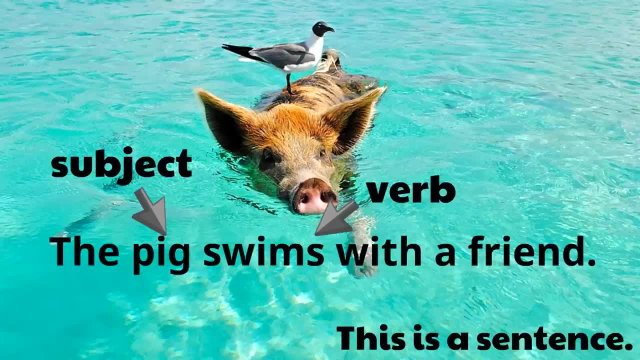 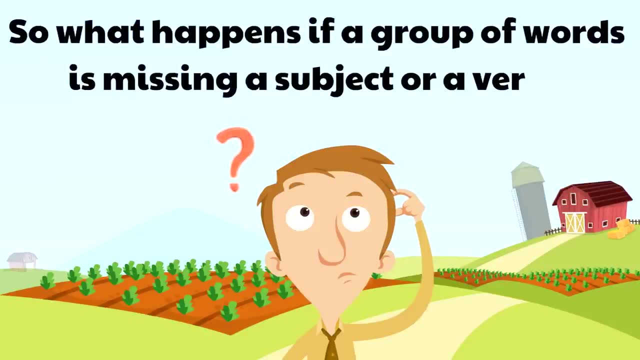 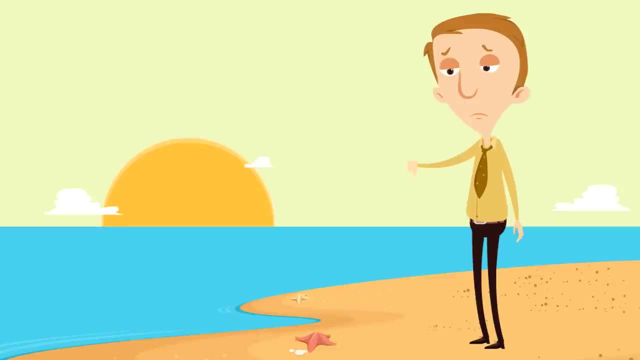 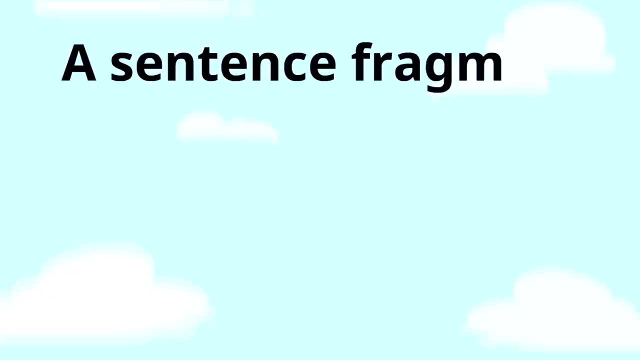 the subject. it's got the verb, it is a sentence. so what happens if a group of words is missing a subject or a verb? well then, it's kind of like me on the beach without my shopping cart. you know it's missing something. a sentence fragment is a group of words. 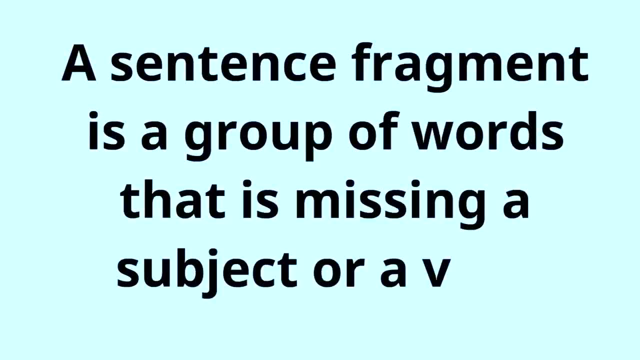 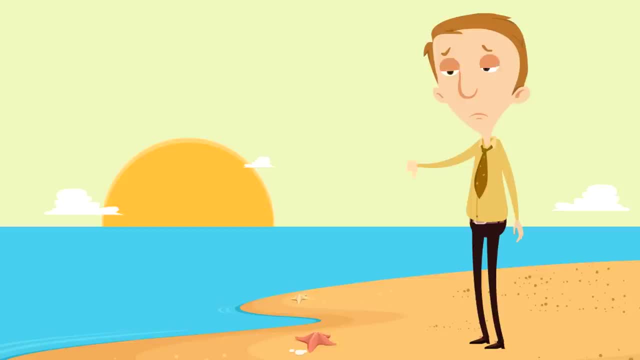 that is missing a subject or a verb. that's what it's called as a sentence fragment. when it's missing something, when it's just part of a sentence, it's missing something. it's not a complete sentence, it's a sentence fragment. kind of like being on the beach without my cards. a sentence fragment is incomplete. 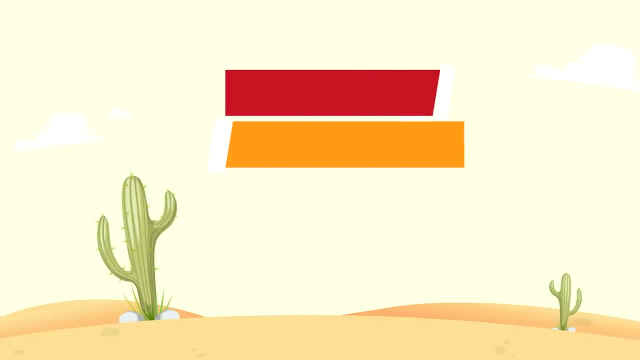 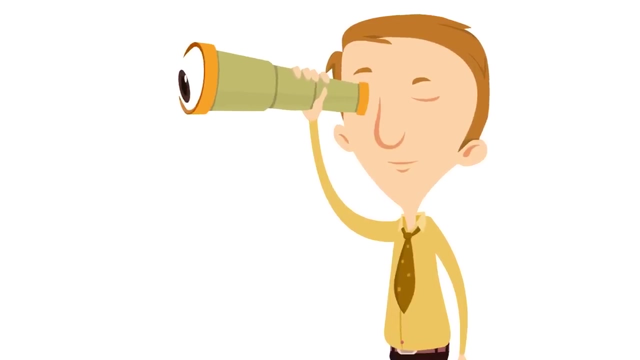 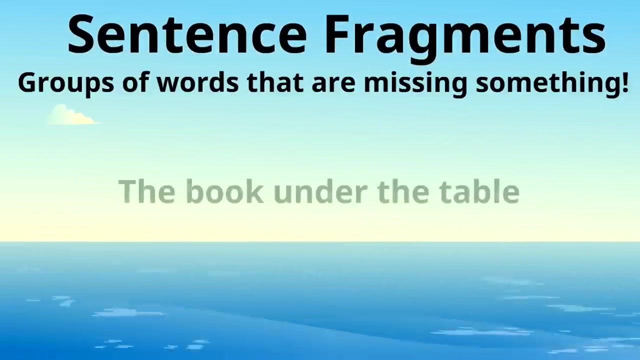 it's missing something. we're gonna show you some sentence fragments so you can see that they're incomplete. they're missing something. they're missing either a subject or a verb. all right, I'm ready to look at them. sentence fragments are groups of words that are missing something like this. the book under the 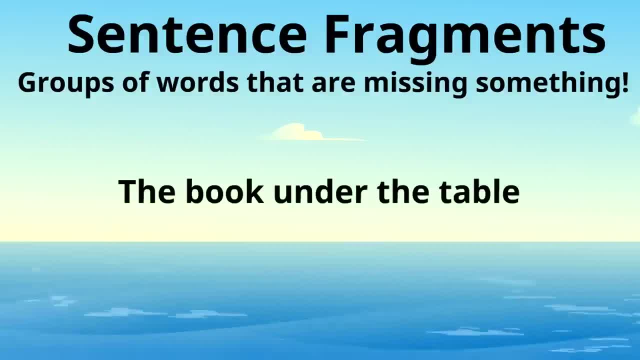 table. what? the book under the table? where's the verb? there's no verb. it has a subject- the book- but there's no verb. it doesn't tell us what's going on with the book. what about the book under the table? there's so many unanswered questions. this is not a complete thought. the book under the 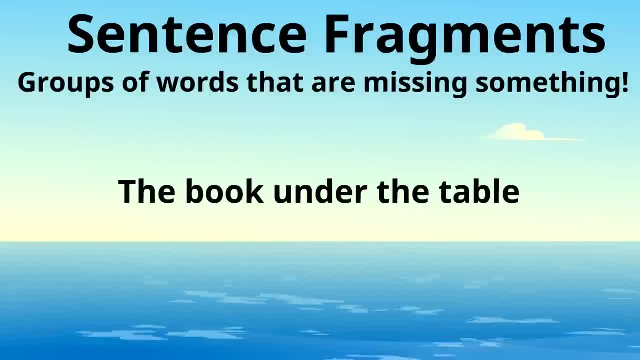 table is a sentence fragment, or how about this? one ran to school. ran to school. it doesn't have a subject: who ran to school? we have so many questions about this. this is not a complete thought. it doesn't tell us who it's talking about. every sentence has to have a subject and a verb. this has the 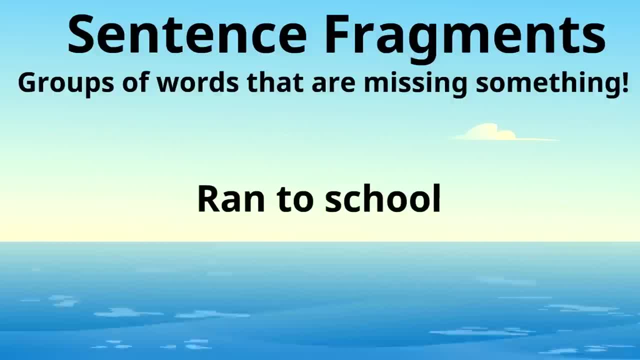 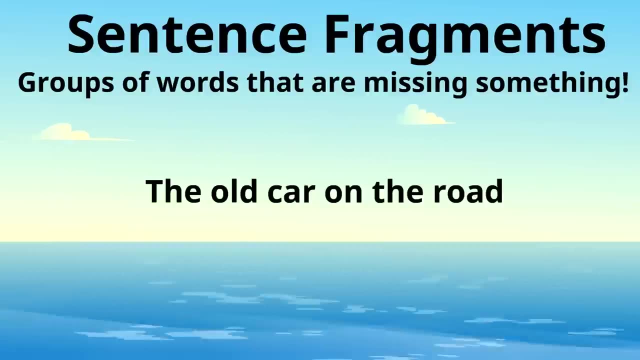 verb ran, but it doesn't have a subject. ran to school is not a complete sentence, it's a sentence fragment. look at this one: the old car on the road. wait a second. this doesn't have a verb: the old car on the road. it's missing something. 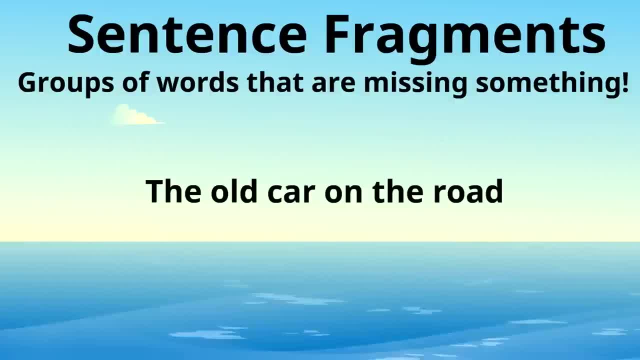 isn't it? it's a sentence fragment. it's not telling us what the old car on the road is doing. it's just saying: the old car on the road. well, what about it? what about it? what is the old car on the road doing? this is a sentence fragment. 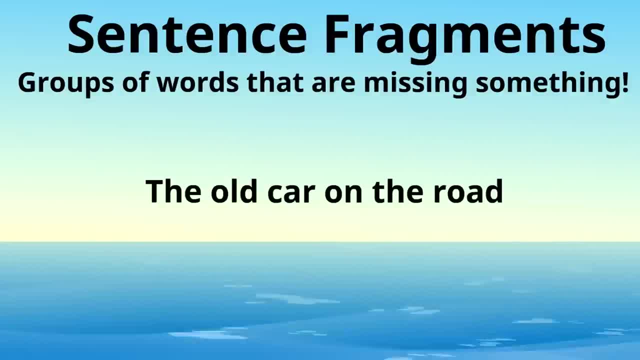 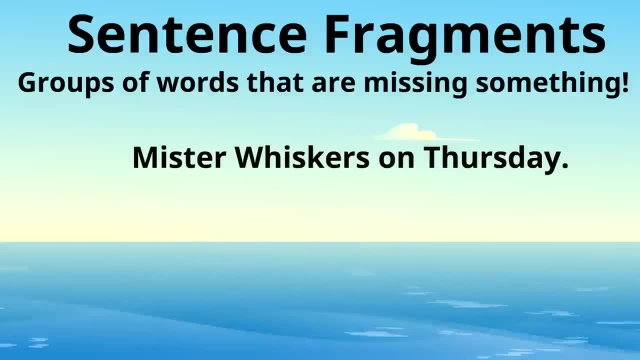 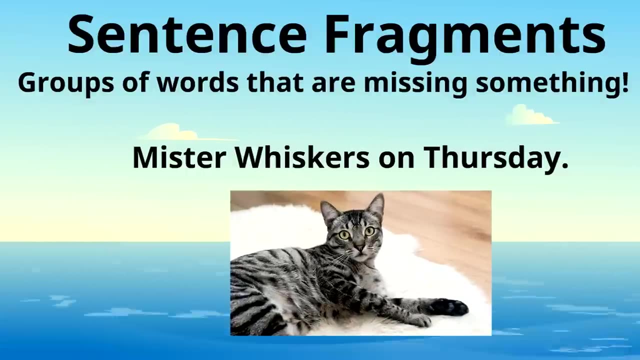 it's a group of words that's missing something and our final sentence fragment is: mr whiskers, on Thursday. wait a second. what, mr whiskers? what did you do on Thursday? it's a sentence fragment. I don't know. I don't know. what did you do, mr whiskers? you don't speak English to. 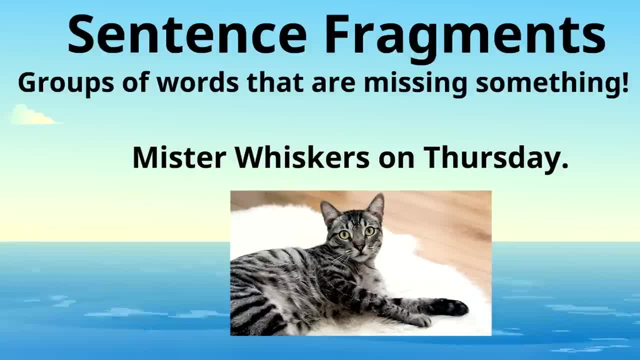 you. I have no idea what you did on Thursday. I hate sentence fragments because they don't give you all the information. there's no verb. I don't know what mr whiskers did on Thursday. it's not a complete sentence. you gotta have a subject and a verb, mr whiskers, please. I hope you enjoyed this video and I'll see you next time. 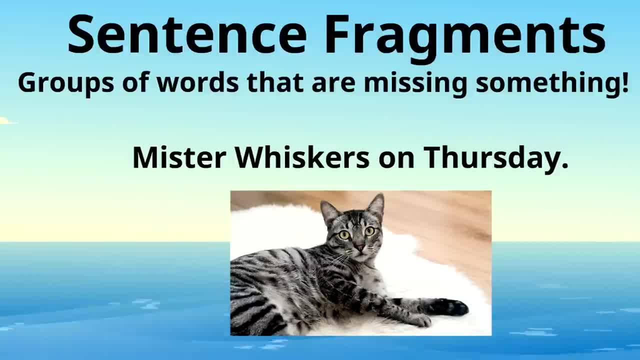 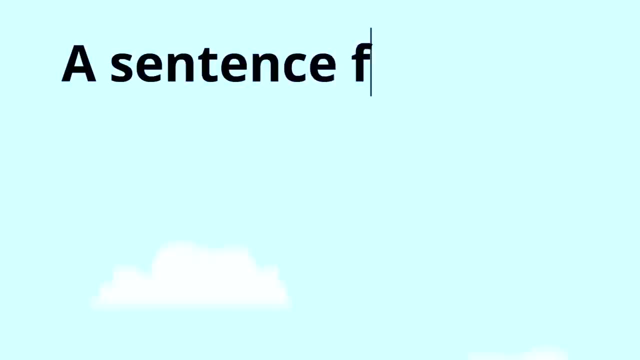 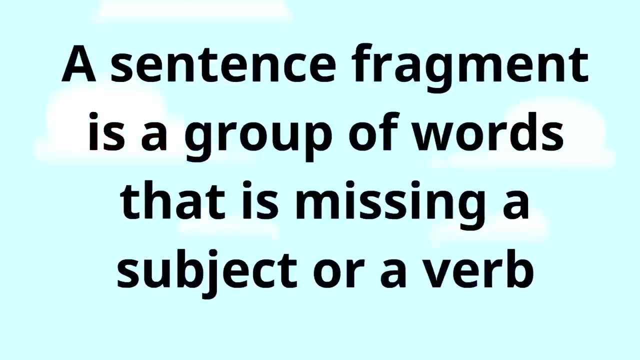 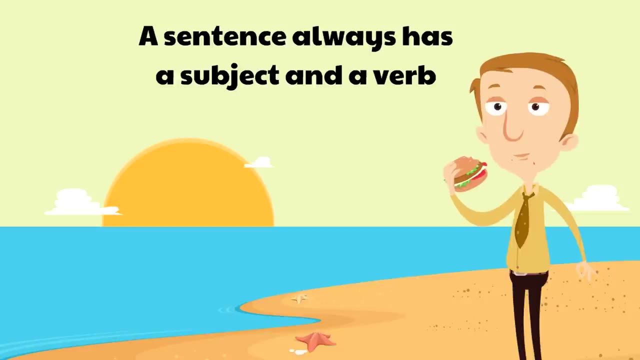 you shave. you know I I go to the beach with my shopping cart on Thursdays and everything to review. a sentence fragment is a group of words that is missing a subject or a verb. now, a sentence always has a subject and a verb. a sentence fragment, though, is missing either a subject or a verb.